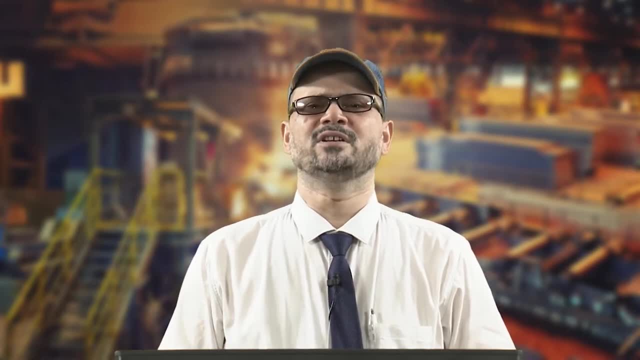 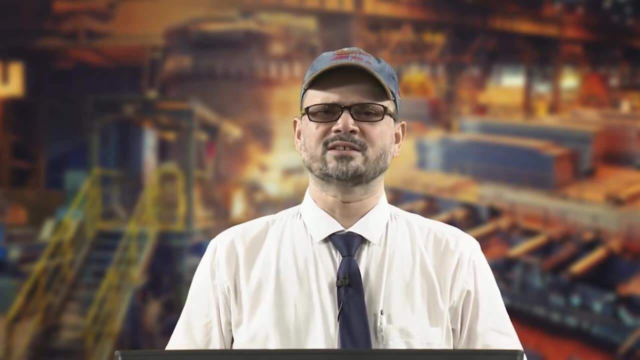 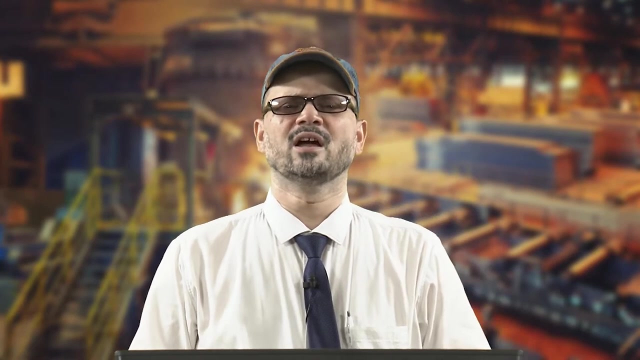 models, then we deal with either the physical model or the mathematical model. Now, in those cases- in the case of physical model, you need to prepare a physical model, which is normally made of you know perspex sheet or so, And then we do the you know physical. 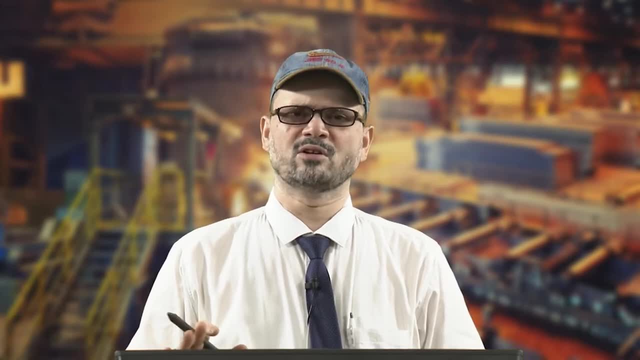 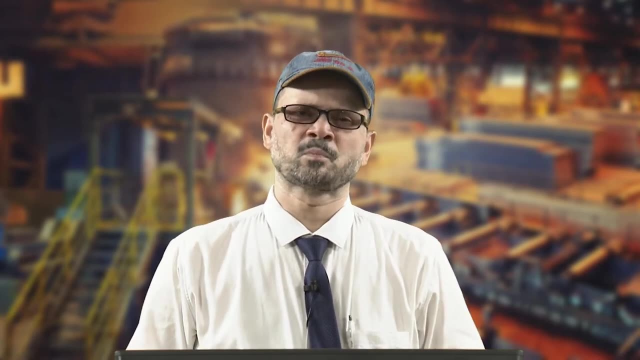 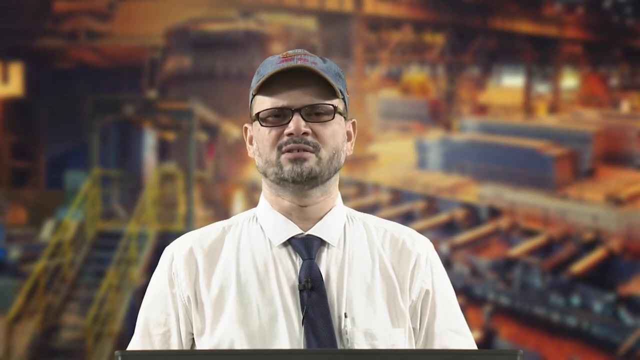 modeling by allowing the water, normally the fluid, to flow, Whereas in mathematical modeling, you know, you know, we have the set of equations. So these are the equations which are representing the case of the phenomena which is occurring inside the Tundish. And then these equations, 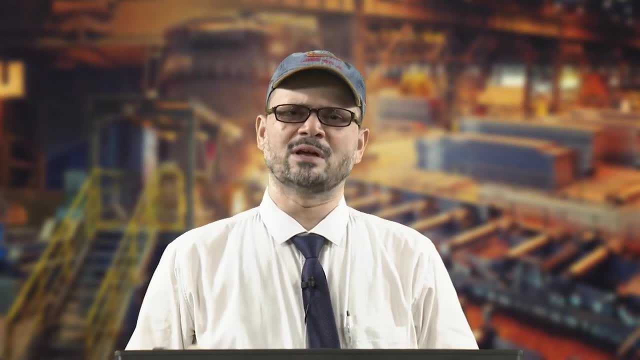 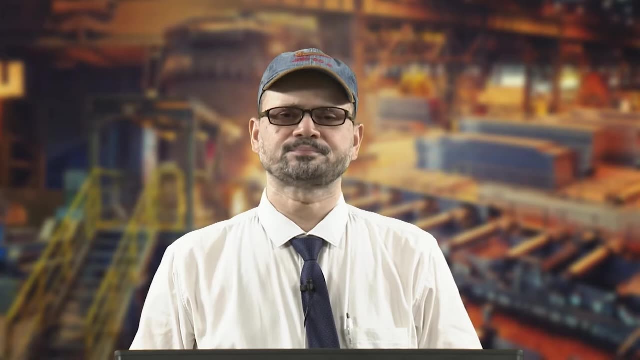 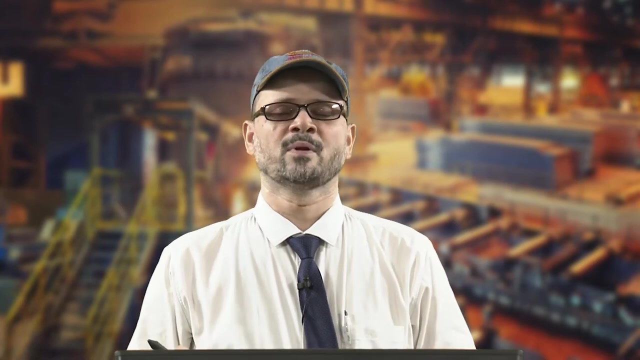 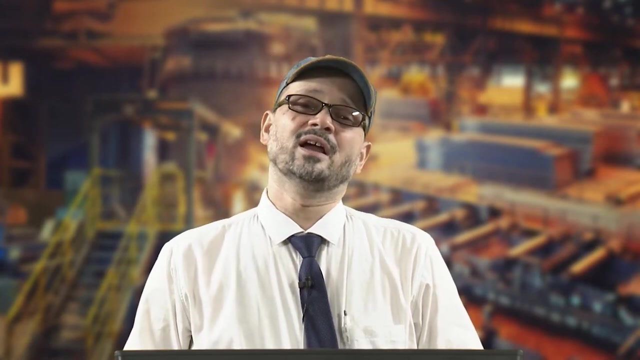 are needed to be solved, and we also have studied that, how you know the the equations are solved and how you get the results. Now, the thing is that, being the era of computers, we normally do the computation on computers, And also for having a better understanding. 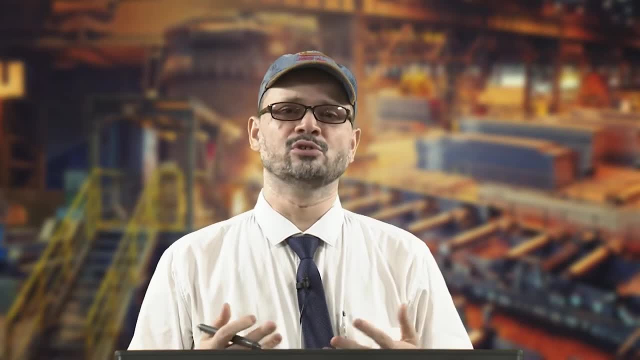 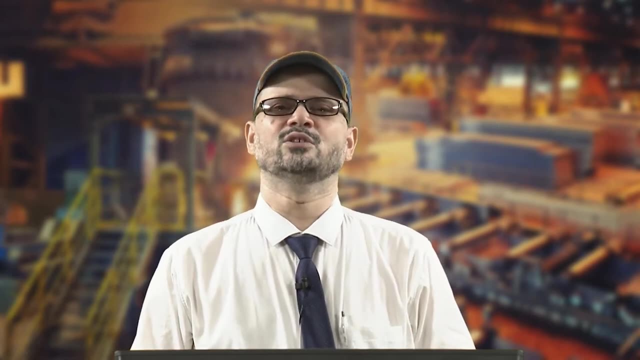 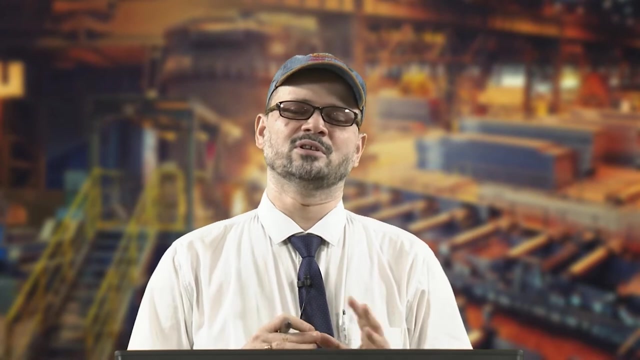 you know visually. we have nowadays tools where you can have the geometric creation. you can see the geometry. then you have to apply the conditions you know. So you have to take first of all these you know conditions, or you have to have the assumptions and you 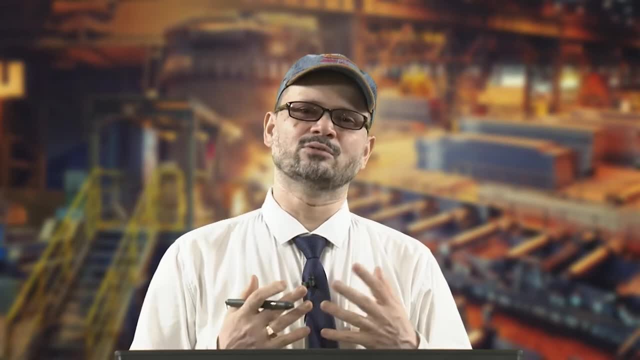 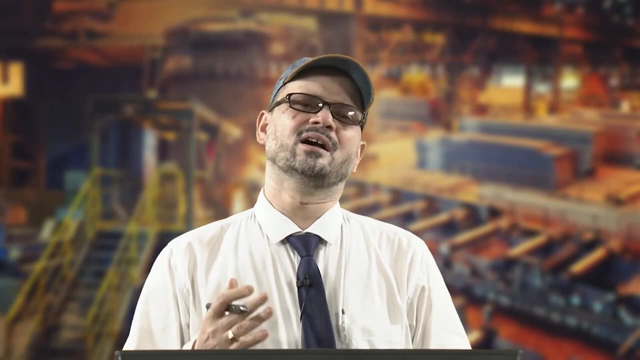 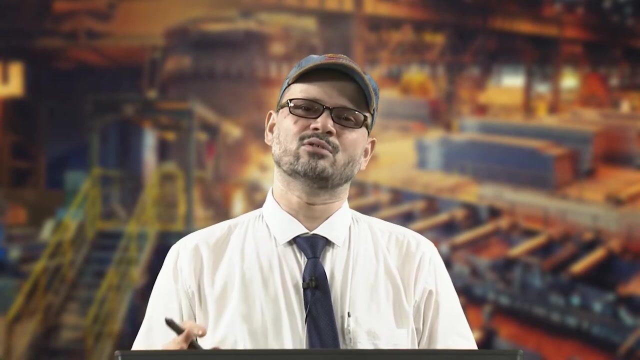 have to also take all the conditions which will say that you are solving which type of problem. Then you are making the geometry and then putting the conditions- different conditions at different places- and then you are solving the equations in that particular domain and then you are getting the results and interpreting them. 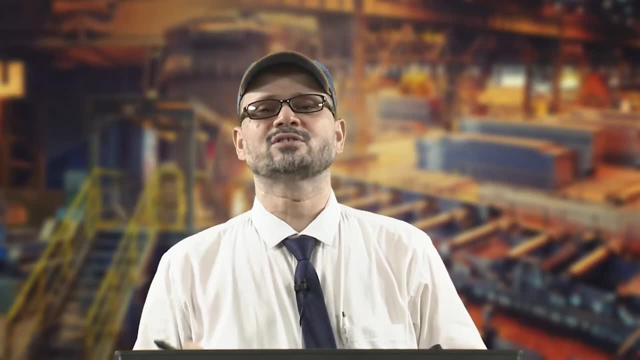 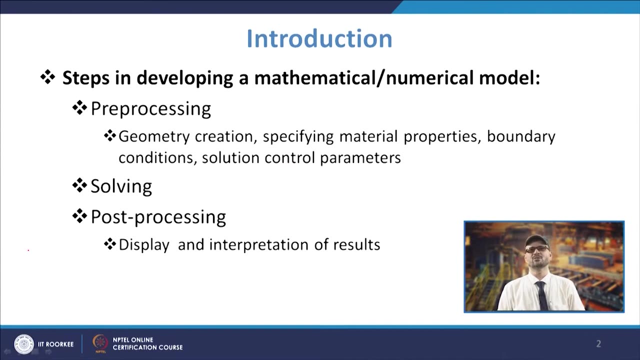 So if you talk about the, you know elements of the model, mathematical or numerical model which you develop towards the. you know flow in a tundish, flow and heat transfer in a tundish. So basically they are done under the. you know three heads. one is the preprocessing. 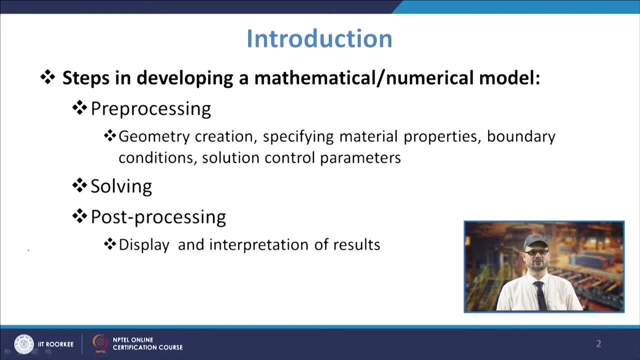 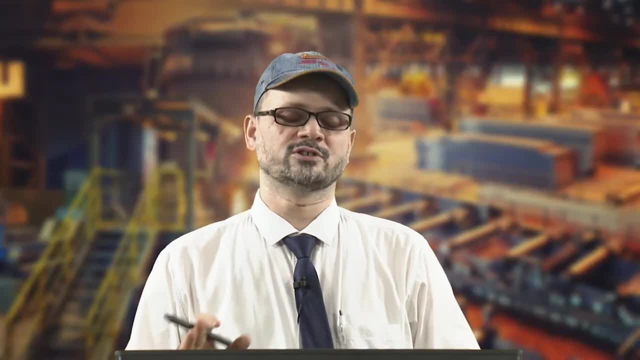 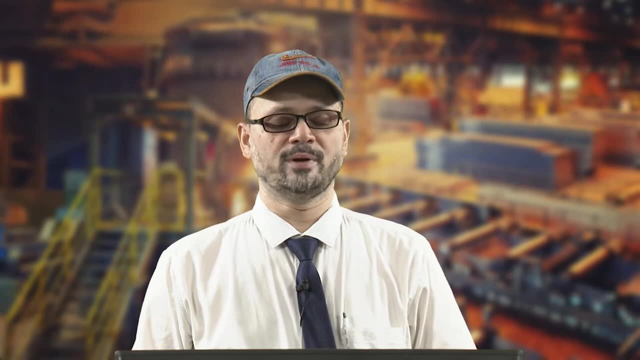 another is solving, and then you have post processing, So mostly the CFD tools. when we use the CFD, you know, do the CFD analysis. So basically our work is divided into these three main, you know, domains. So preprocessing, solving and post processing. 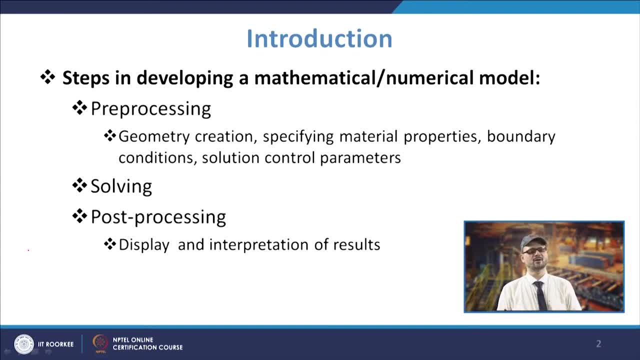 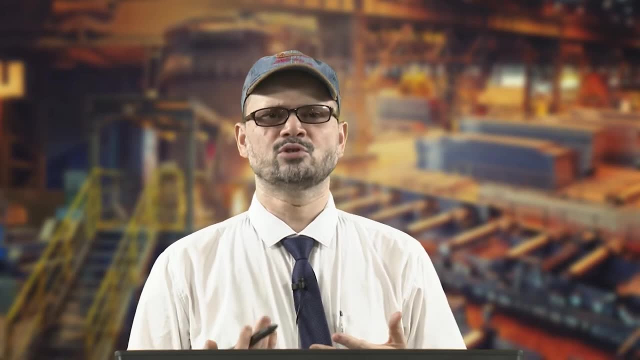 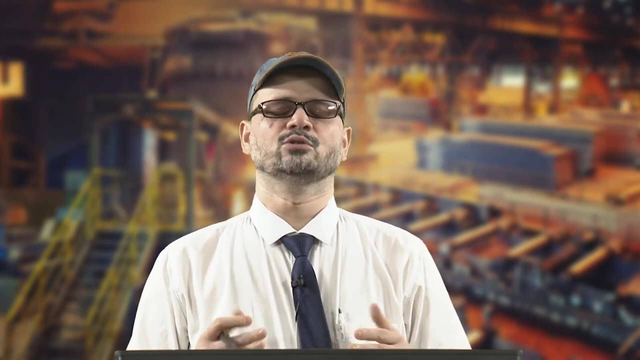 Now what we do in preprocessing the? in the preprocessing we do the geometric creation. So normally what we do is We have to create a particular kind of geometry So that geometry will be available to you. if suppose you are making the model of the tundish, So you have to make a tundish using 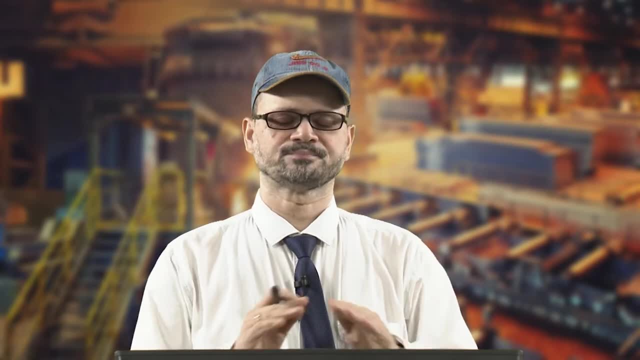 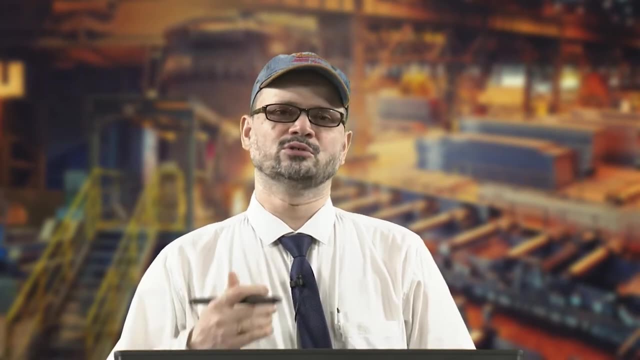 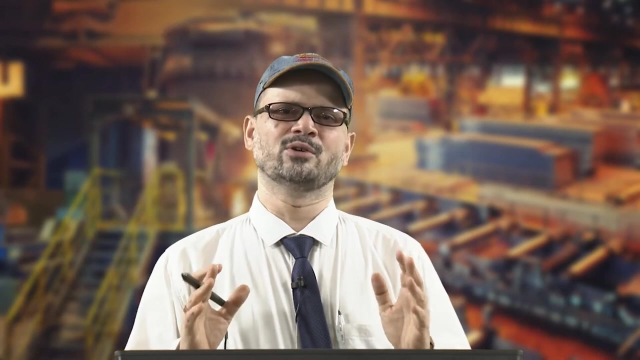 a using a tool which, So by which you can create the geometry, and that we will discuss that. how you know, you create the geometry, there are many approaches by which you create the geometry, So that geometry, you know, has to be there with you. In normal case, if you start the 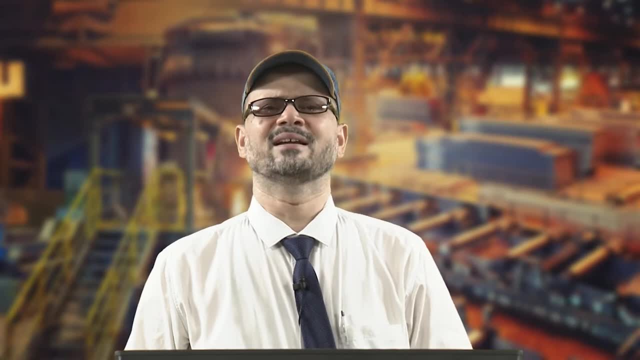 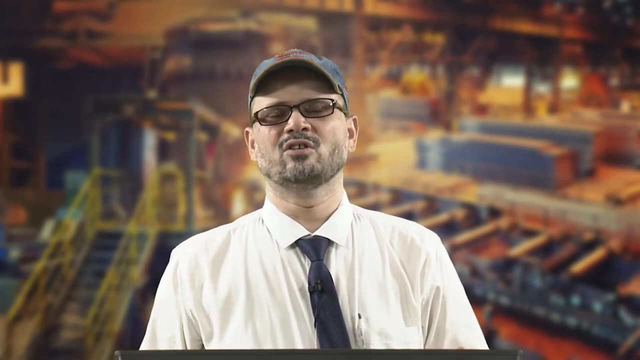 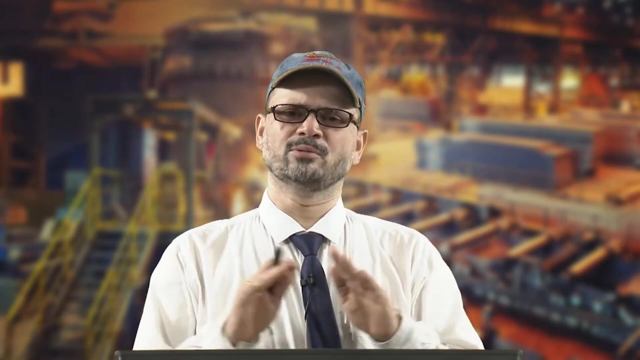 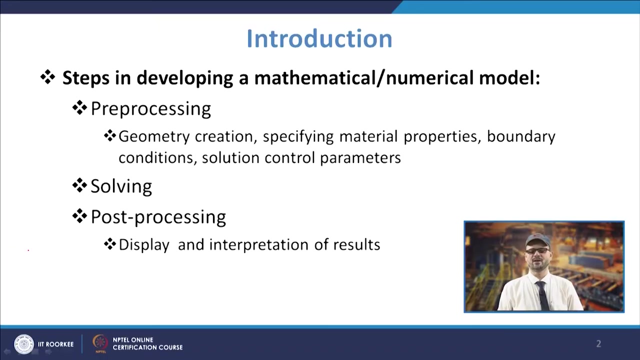 simple. you know analysis. you can have a geometry of rectangular shape of box if it is of three dimensional, or you can have a two dimensional geometry also, So that geometry needs to be, you know, clear in your mind Then. So what you do is you specify the material properties. you know material of the you know. 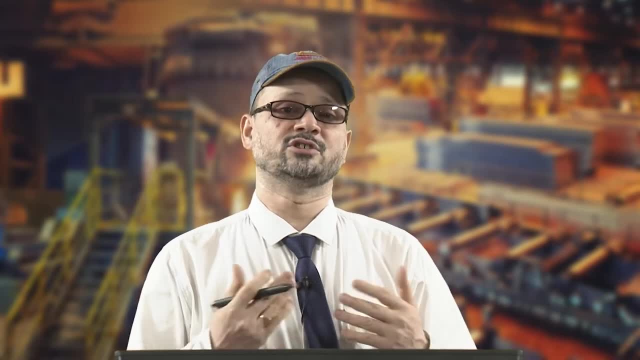 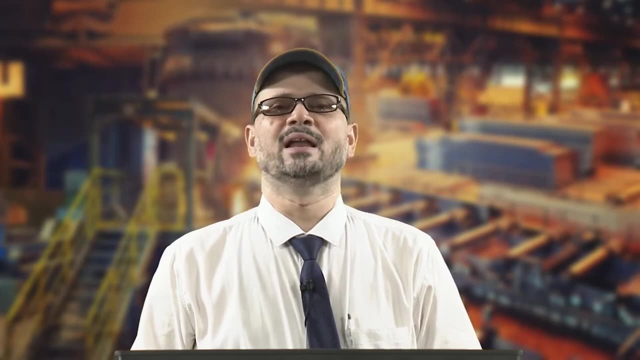 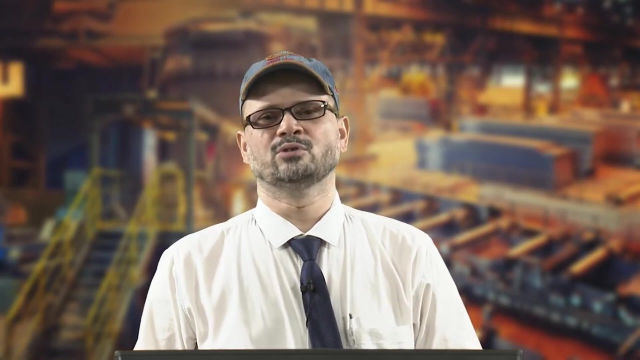 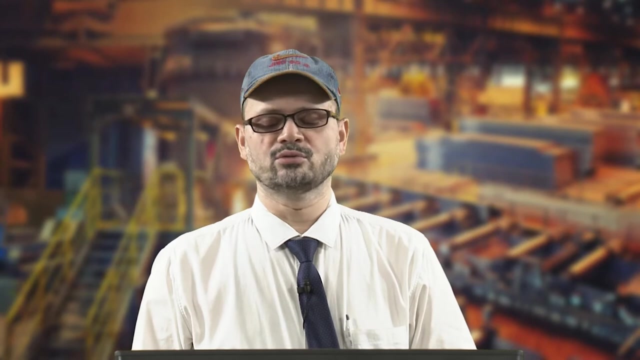 tundish by which it is made, or material which is going to flow inside the you know tundish. So you will have the boundary material of the walls, or you know the material of the prop, the steel which is flowing inside. then you are going to impose the boundary conditions. 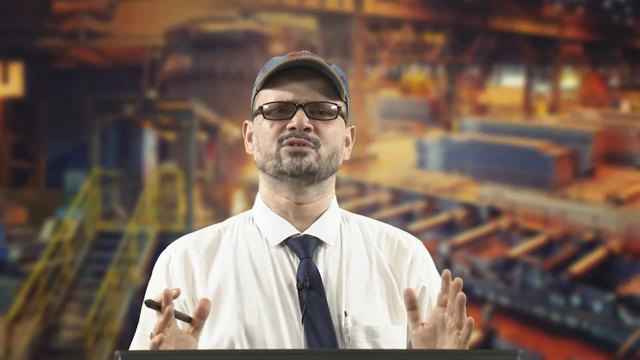 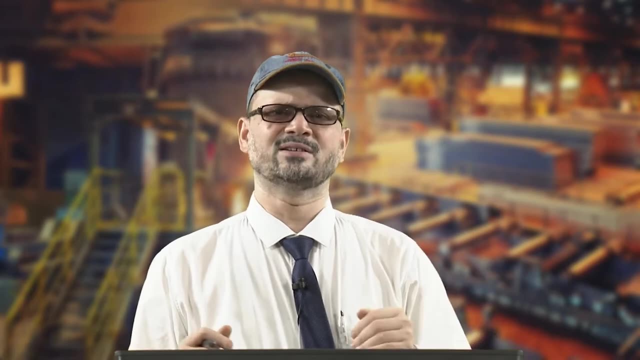 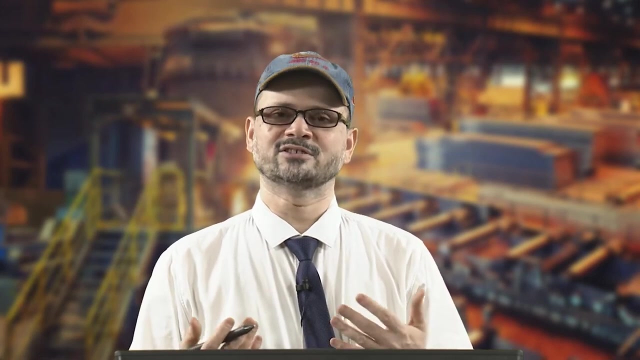 So boundary conditions will be there, those conditions which are specified on the boundaries. So boundaries are especially the walls or the inlet or the outlet. you may have blocks inside, So, and you will have a boundary conditions, maybe of different type, you may have the boundary. 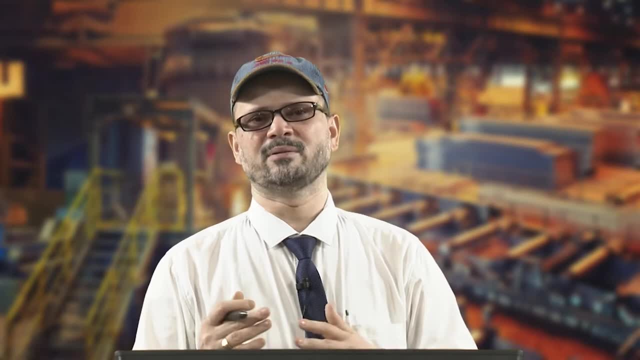 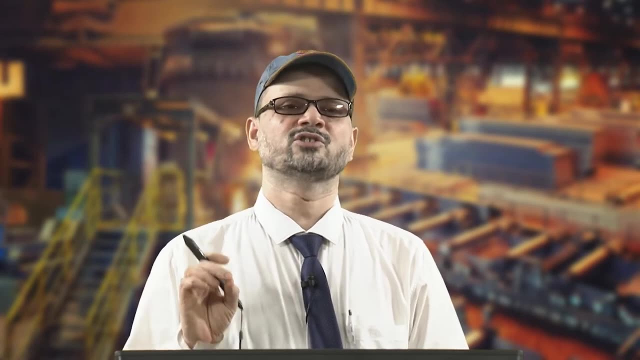 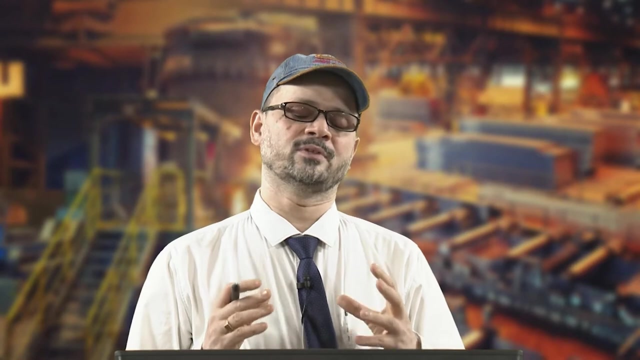 conditions. It may be related to flow, it may be related to heat transfer, it may be related to pressure. So there may be different kind of boundary conditions which you need to specify in the domain, and then you are going to have the solution: control parameters. 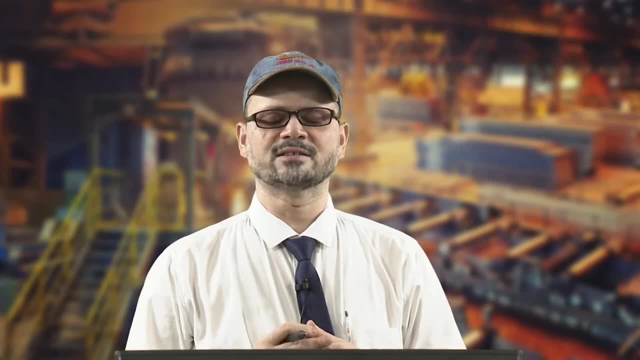 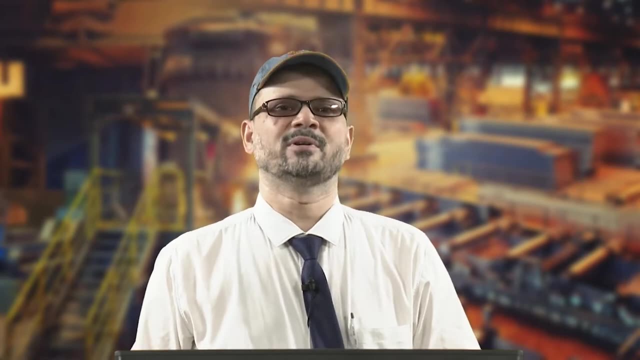 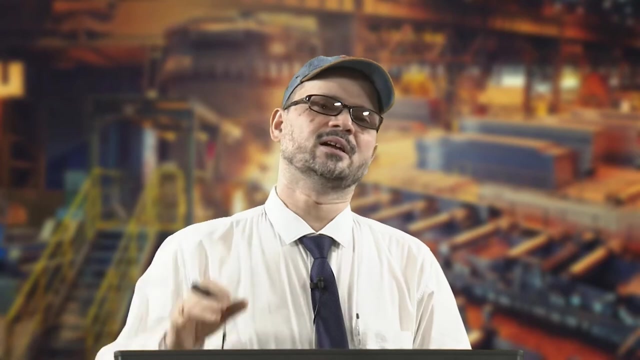 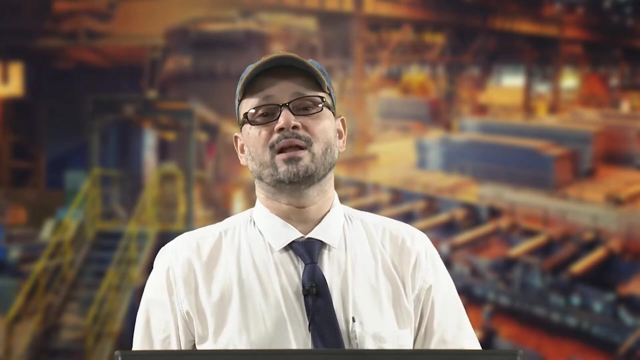 So once you put these boundary conditions, you specify different zones as the walls, or you know the Symmetry or the, you know periodic boundary conditions or so, or you specify the inlet and outlet and other all other things. Then after that you have to go for the solution, control parameters, you have to provide those. 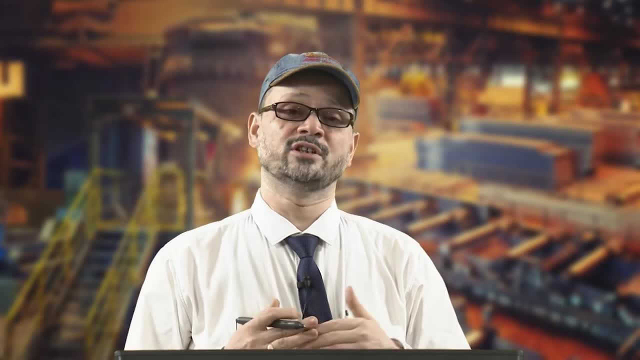 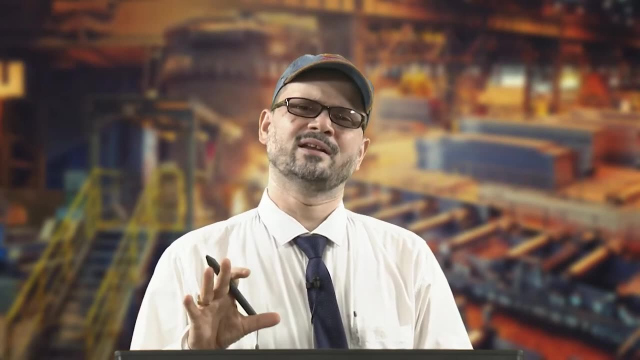 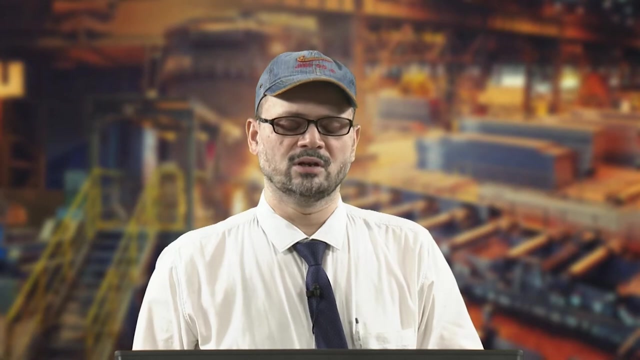 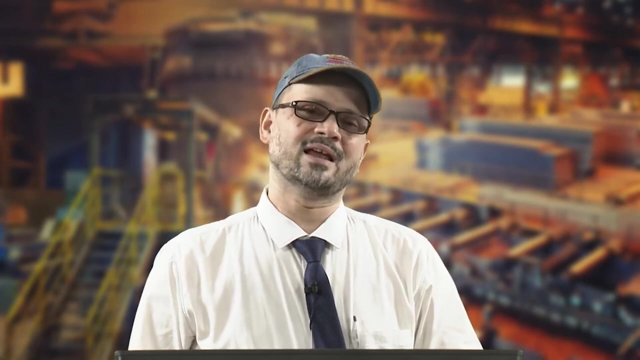 parameters, which will be talking about the solution which will be done. So, basically, there, you need to provide, you know the number of iterations you want to do. Then you have to go further, then you have to, you know, specify the time step size if you are going for the. you know the transient type of analysis. 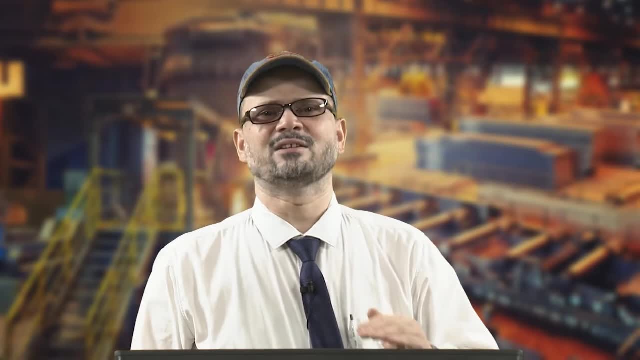 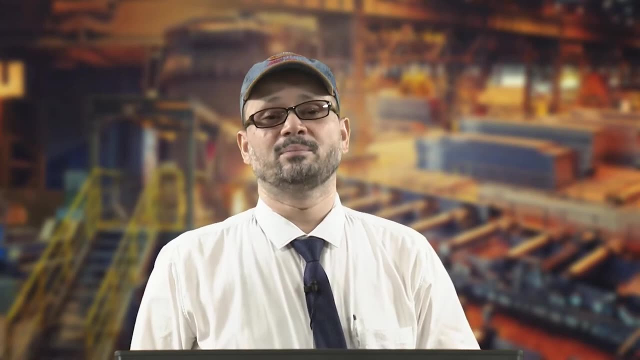 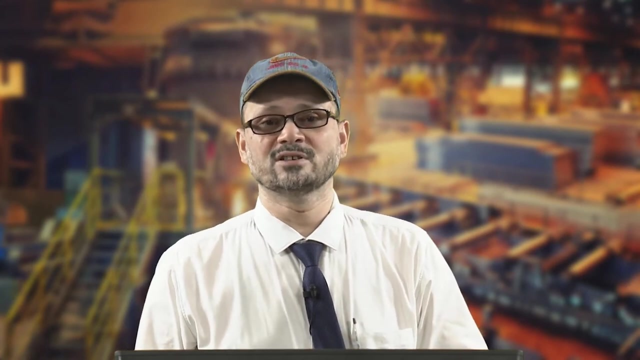 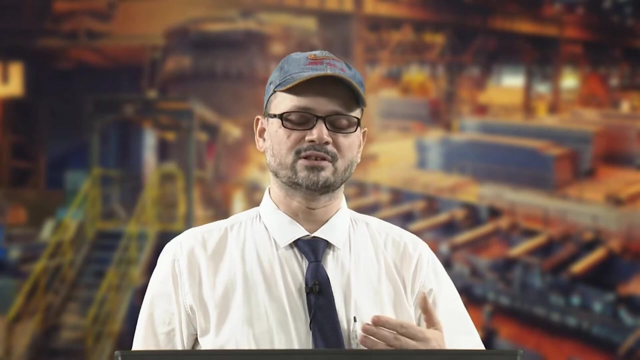 So you will go for the you know time, step size that will be provided. Then you will also go for the you know parameters, which will be helping you in getting the solution converged quickly. So that is it, Thank you, And give you the meaningful kind of results that will be the relaxation parameters. 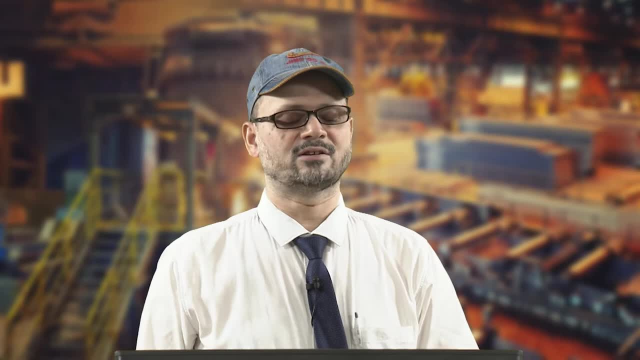 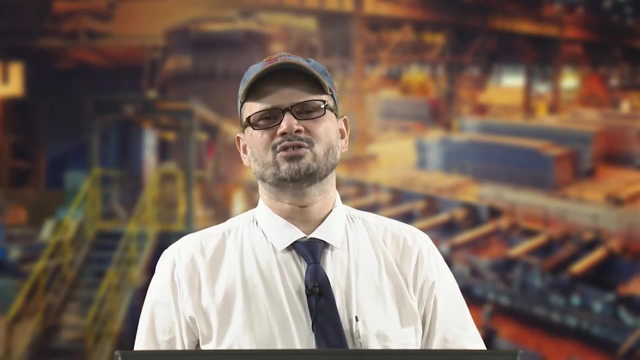 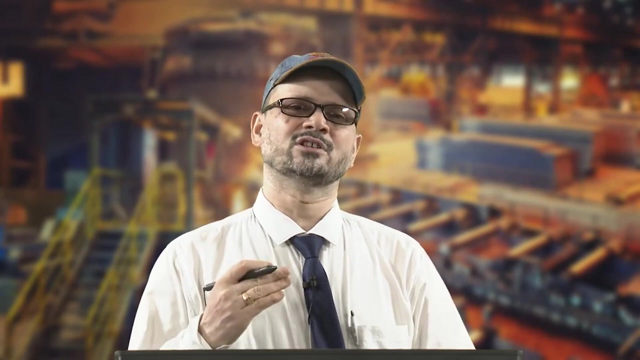 So those parameters will be, you know, under that solution, control parameters. Now you have to go for this solving And solving. most of the tools may have a separate solver, So that will ensure that the equations which are there integrated because of the type of 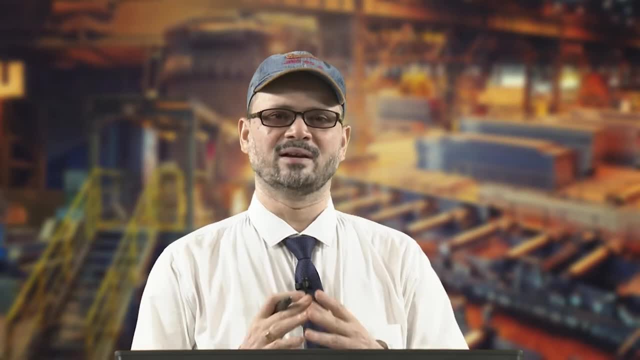 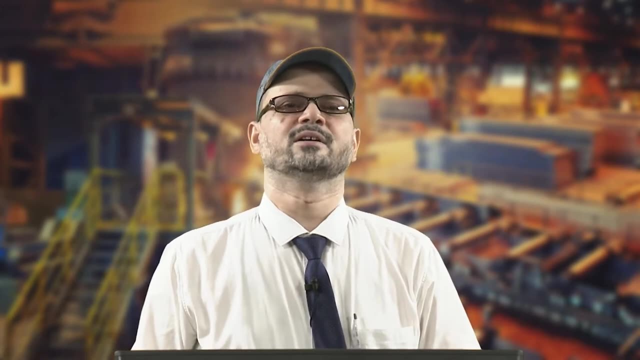 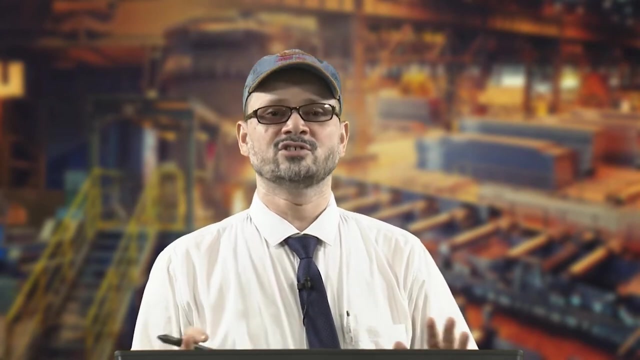 problem you have taken and because of the conditions which you have given. So ultimately they will be resulting into the set of equations and these equations, typically, if you are solving, you will have Navier Stoke equations, you have the equation for energy and they need to be solved. 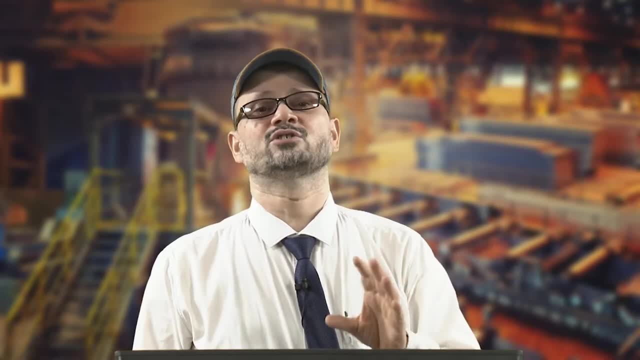 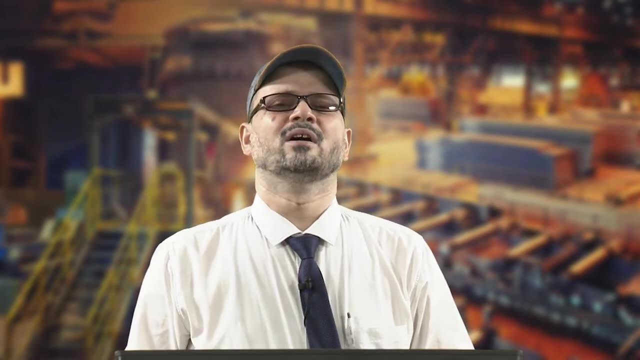 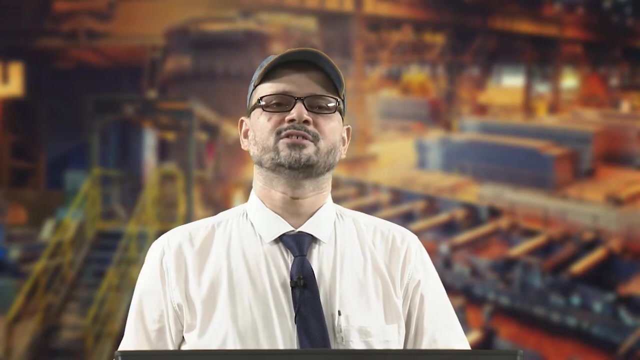 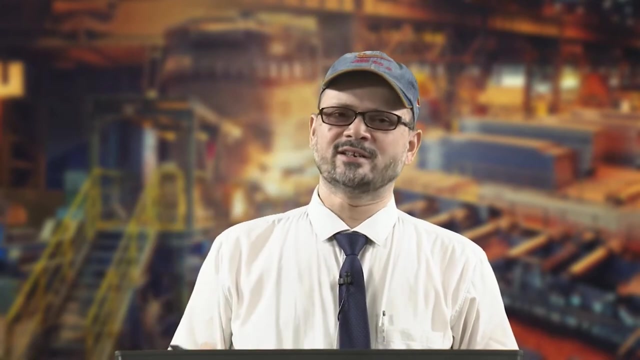 And then they need to be solved using this solver. So you may have the solving option also and you will be solving these. So that will run. and in case of the steady state- you know type of the problem- you will wait till the steady state is reached And then you 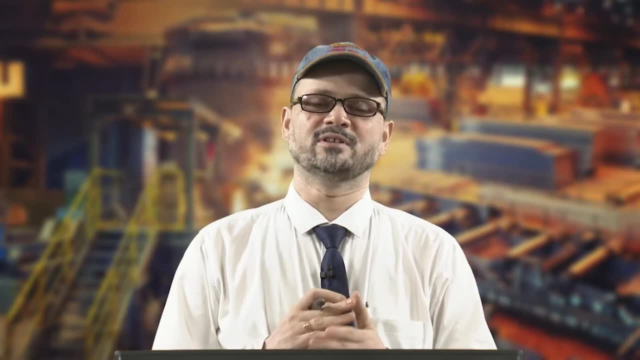 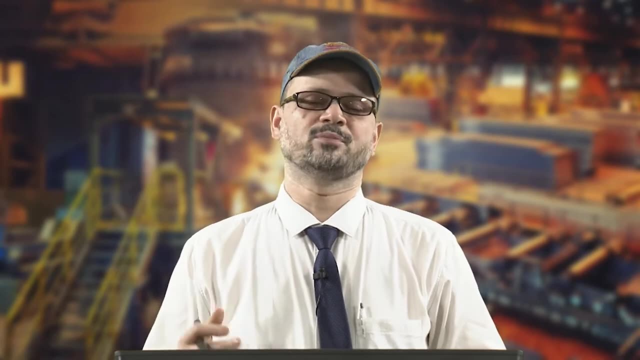 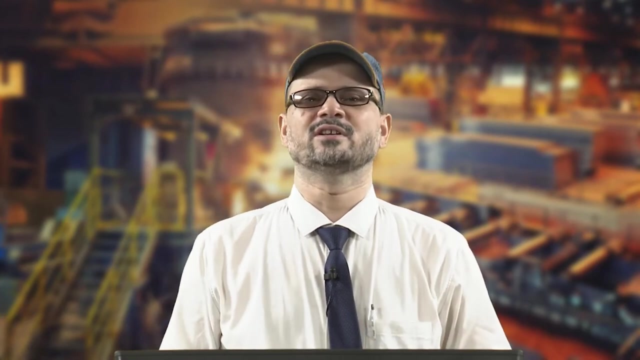 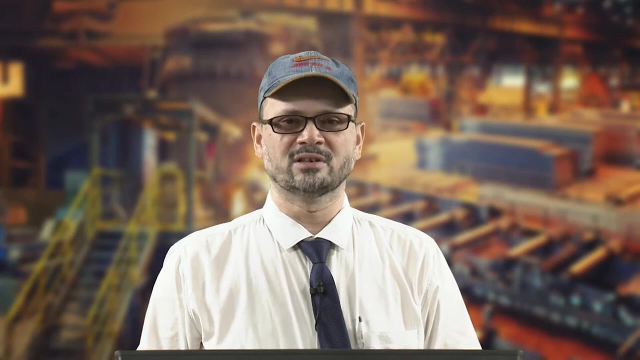 have also many a times problems like the in case of transient. you will see that the how you know with step size, that iteration Go away, go forward and then when the you are at a stage where the solution is solving process is over, then you go for the post processing operation. So in the case of post processing, 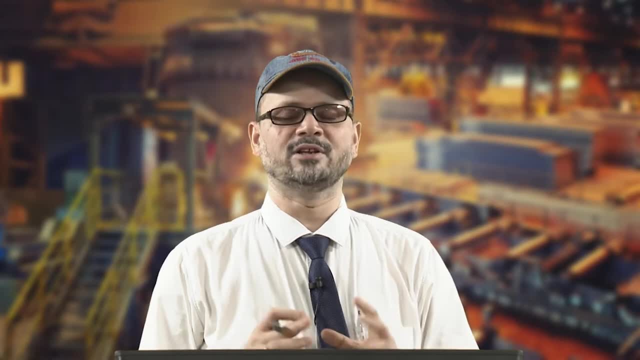 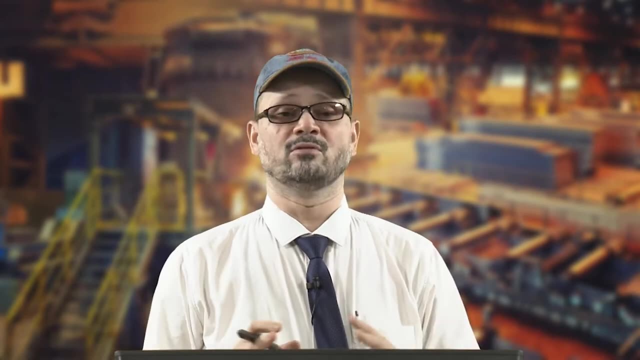 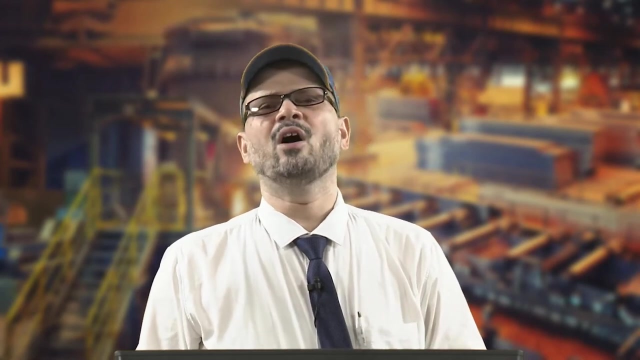 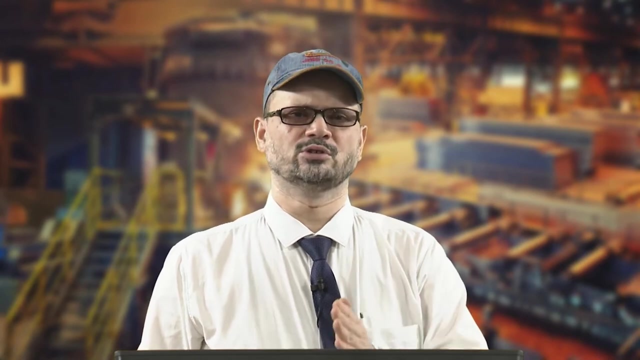 operation. you are going to have the analysis of the results, So you have the visual display of the results- And to have the- you know- velocity or the pressure or the or computation of any parameter. you know that we try to find and that is known as post processing. So post processing means: 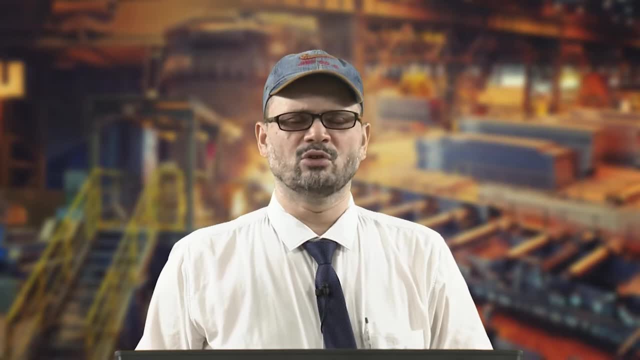 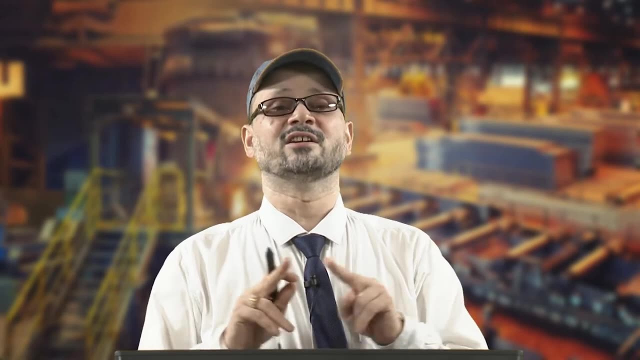 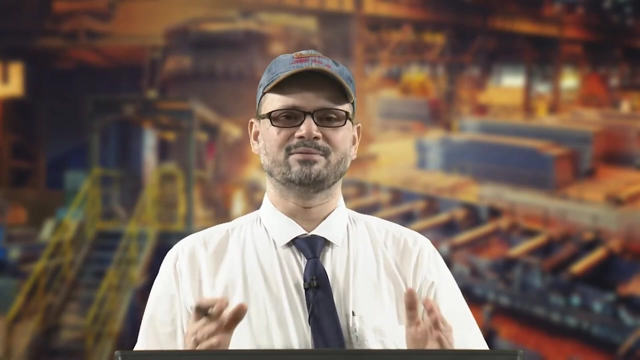 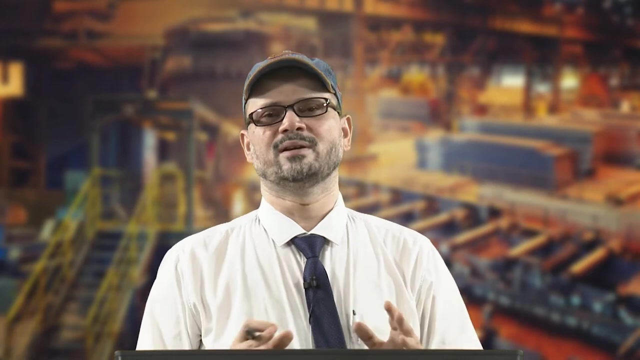 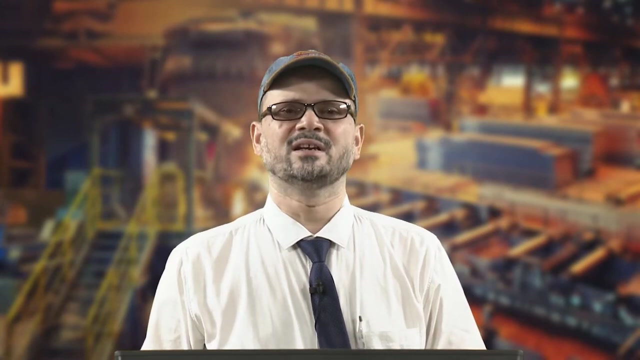 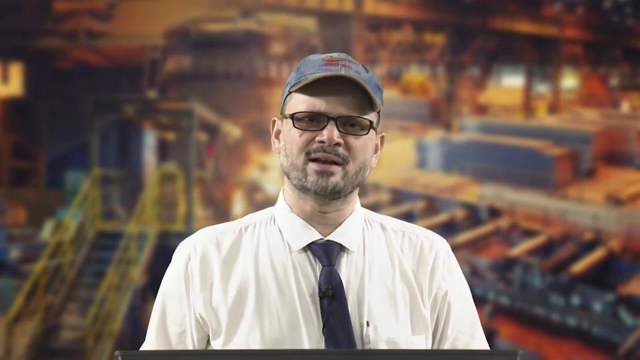 after the solution is over, after the solver has done its job, then you try to further see the results. 你能得到正確的結果. This p is interpreted in a proper manner, so that you get the meaningful results, So that 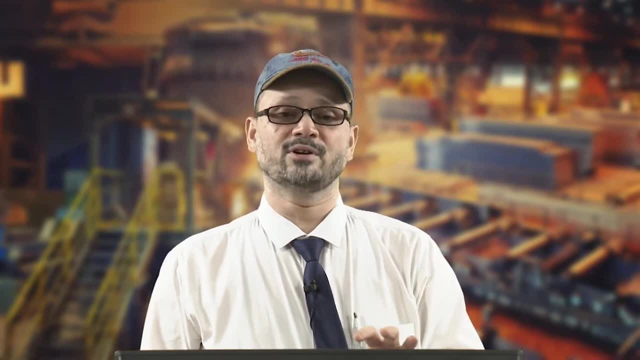 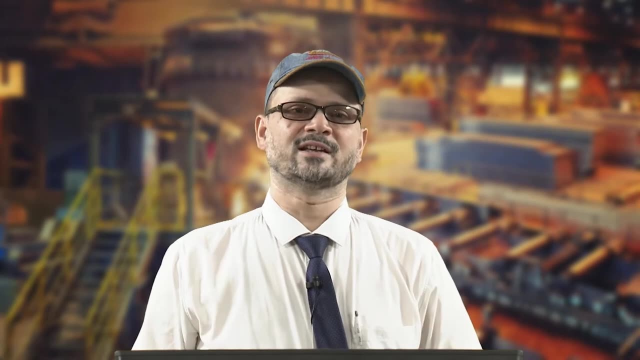 is why post processing also is important and there are tools available which will properly, you know, show quickly, it can show you the graphs of or relationship between the different, you know, operating parameters And then, accordingly, you can have these interpretation of Werk ragel ou ga Legend: Vanill snack. 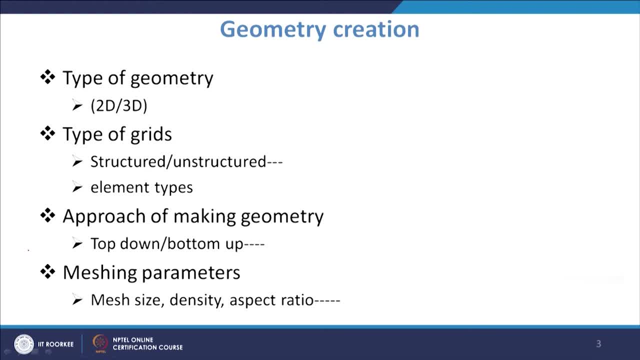 No, the entireUmphyRawRawRawRawrRawRawRawRawRawRawRawr Anfang the results. So now we will go towards the geometry creation, which is the initial step. you know the first step, because you know, first of all, you need: 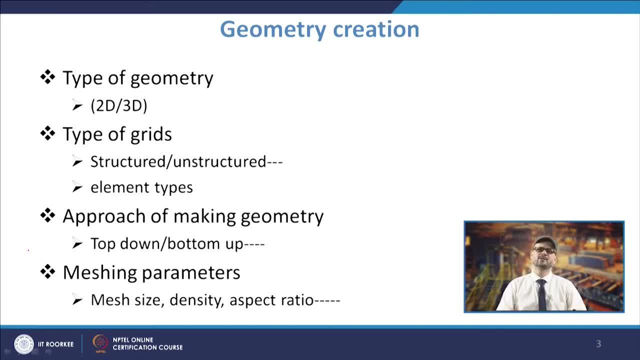 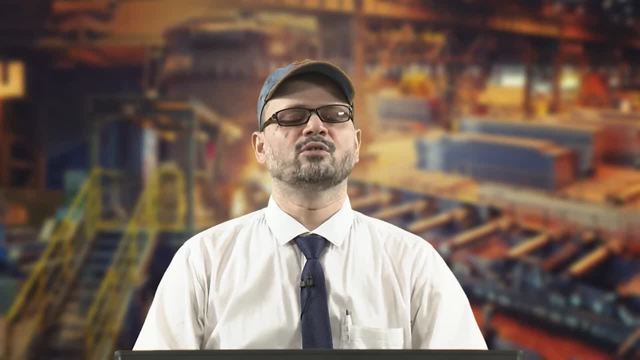 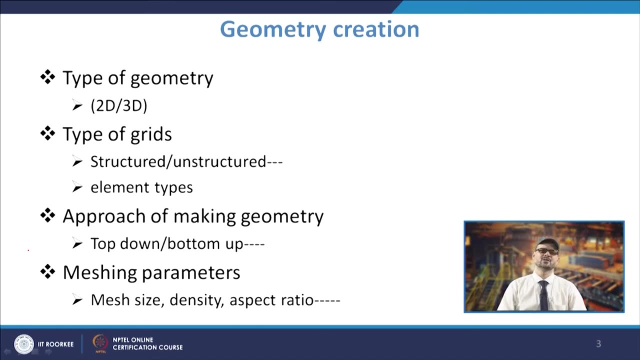 to have a proper geometry of the you know, the tundish or any vessel which you are making. So you have to decide: we are going for the 2 dimensional geometry or 3 dimensional geometry and in that case you will have you know. in the case of you know, depending upon the type, 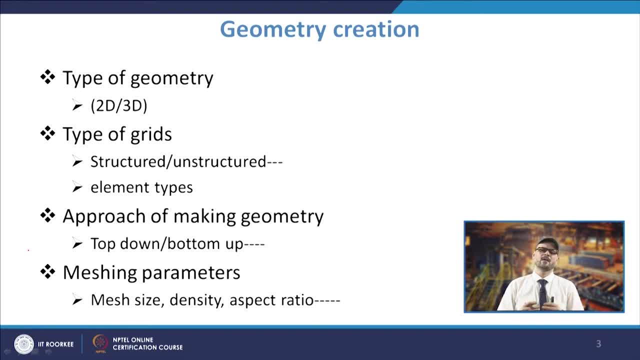 of geometry you will have to choose, because if you go for 2 dimensional geometry, which will be enough for the complete representation of the flow behavior or the behavior of the system, In that case you prefer to go for 2 dimensional geometries because that will 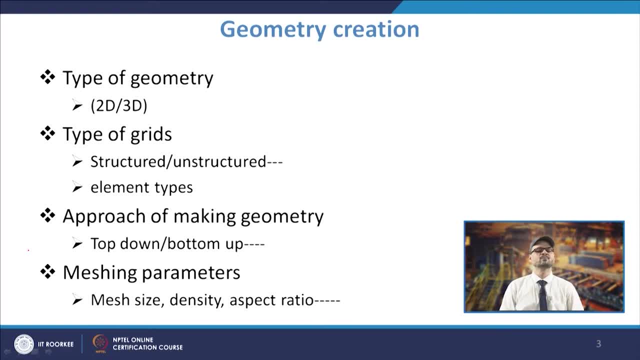 take less amount Of computational time, else you have to go for the 3 dimensional geometries. and then you know the geometry needs to be, you know, divided into small elements and, as we have studied that, you need to apply the these conservation equations So you will have the suitable. 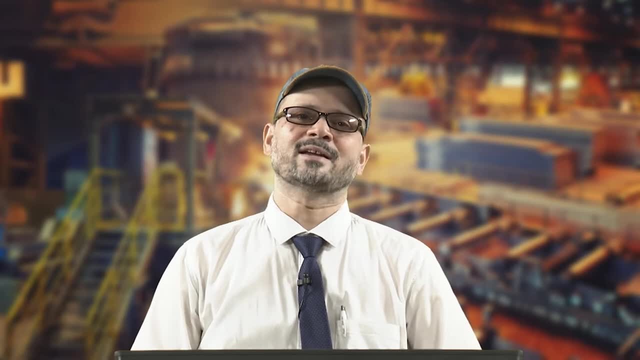 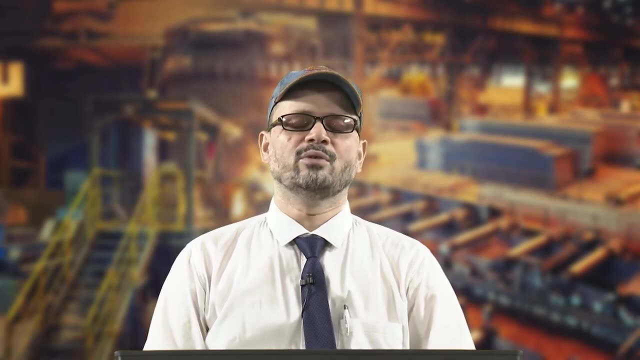 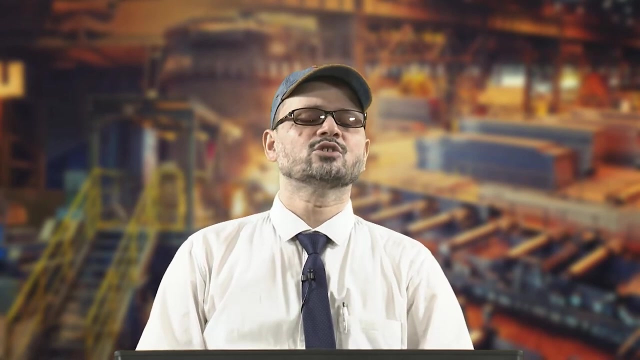 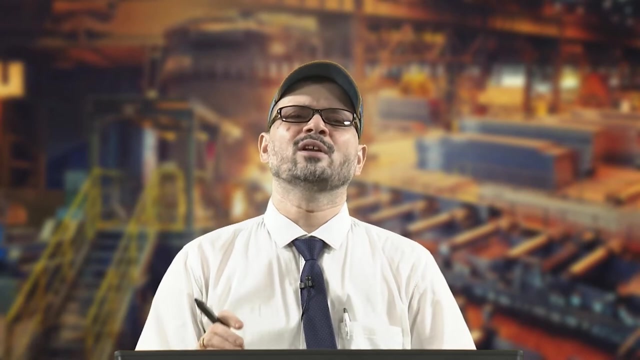 equations, You have the algebraic expressions. basically you get out of, you know out of these conservation equations when you apply the different kind of differencing schemes or discretization schemes. So basically you are, you know, converting the whole domain into small elements, and then 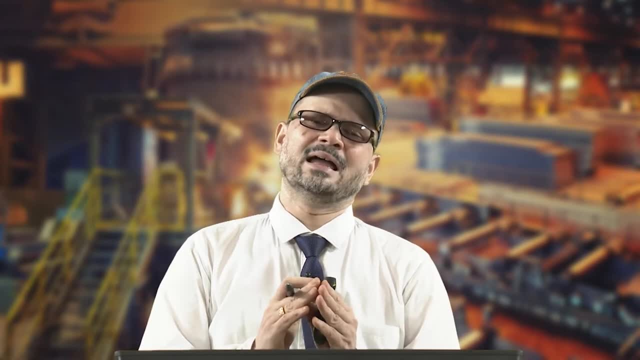 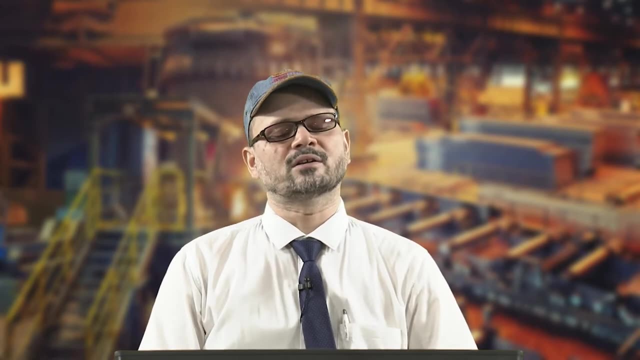 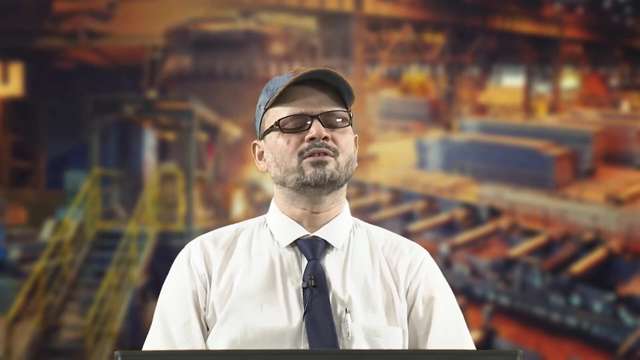 you are. So basically, you will have Divide the domain into different control volumes and then you are going to start the work. Now, as far as the grids are concerned, if you have to know that, what kind of analysis you are going to have on the, you know, on that particular geometry, So whether, depending 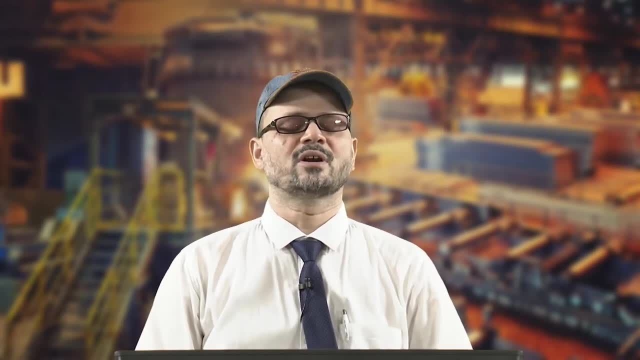 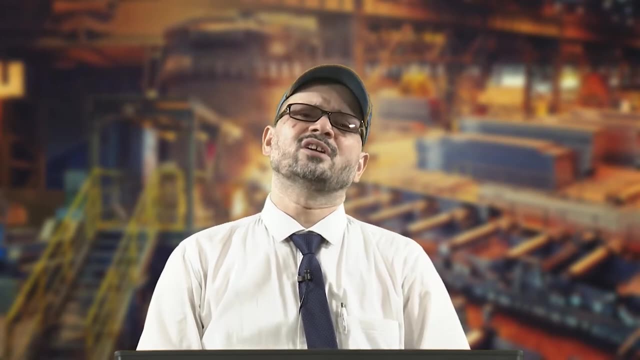 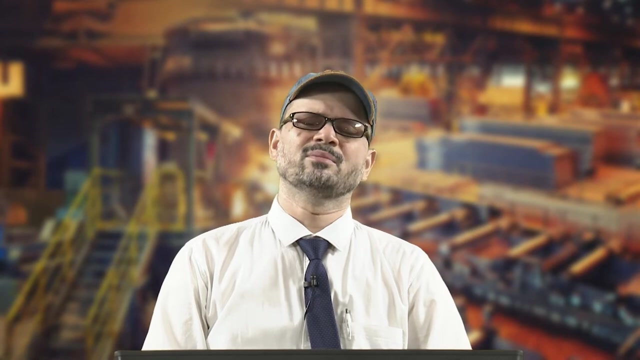 upon the geometry. you have to see that whether you are going for the structure type of grids or you have, So you have to go with the unstructured type of mesh. Now structure type of mesh are there where normally you know you can identify the adjacent cell with the help of the i, j and 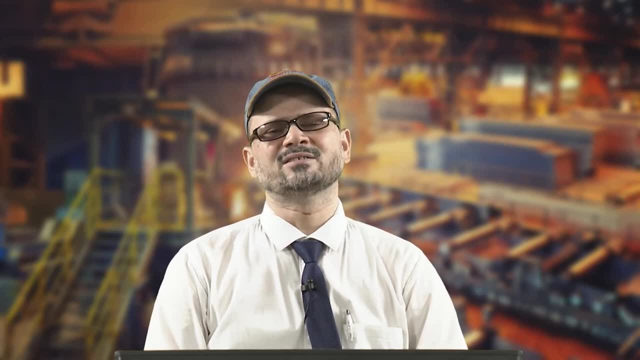 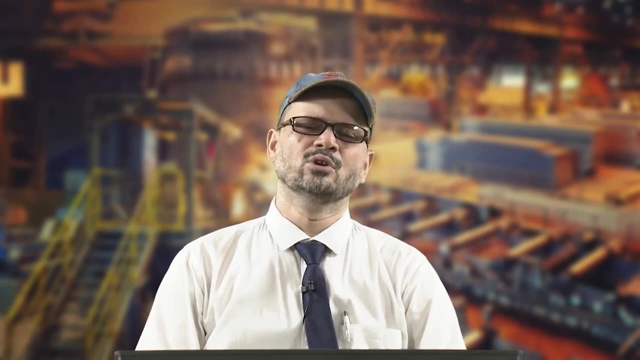 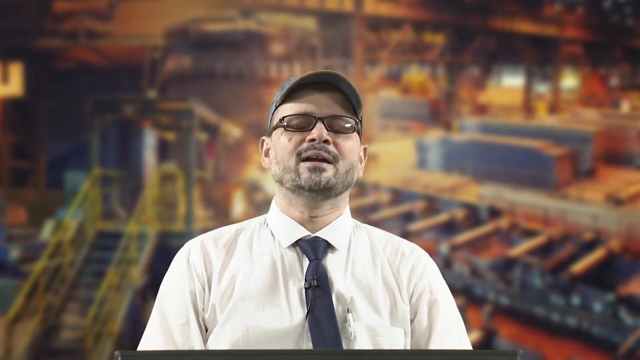 k values. If you are going for the 3 dimensional analysis, in that case, if you have to locate a particular cell that can, that can have a unique i, j and k value. So that is So. that is normally the structured kind of grid and if you have the grid, you know where. 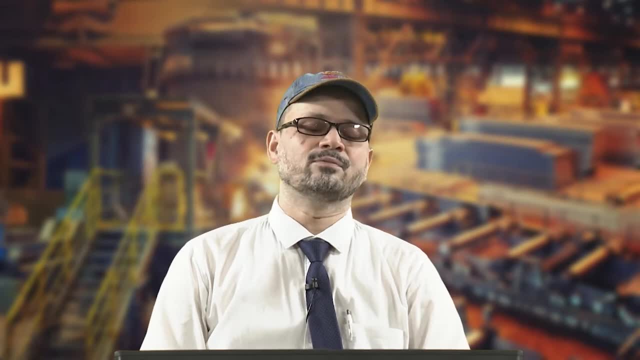 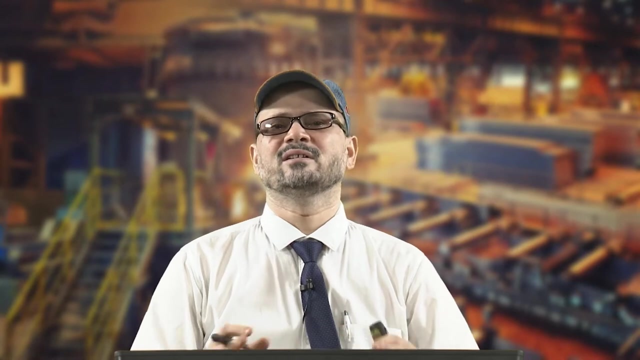 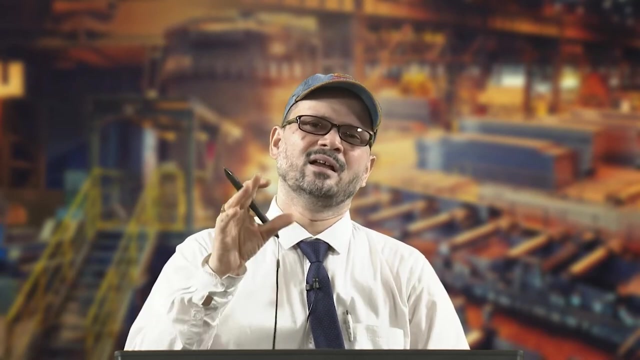 it is not possible to have that kind of, you know, grid structure. So there they are known as the unstructured grid. So in that case, certainly it uses its own internal data structures, its own internal programs and with the help of that It will be taking, you know, you can go for a particular point or on a or a plane, can. 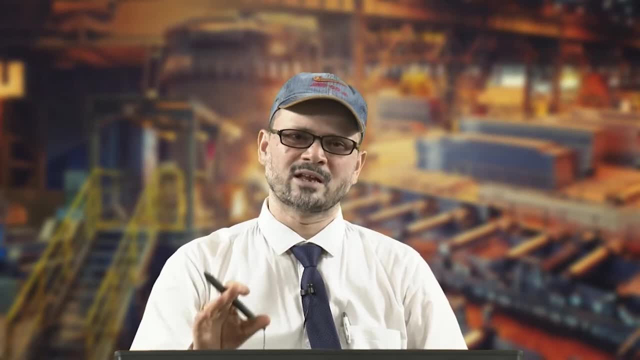 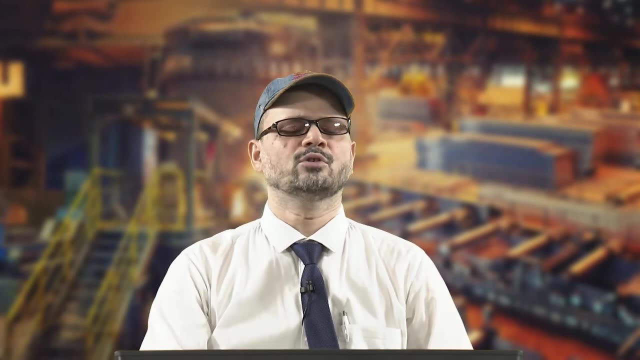 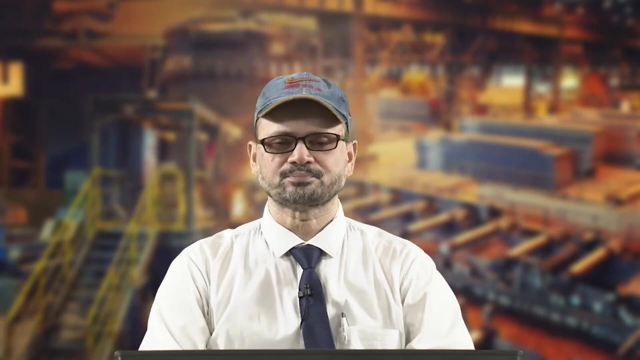 be located, a surface can be located or a volume can be located and accordingly the analysis can be done. So you can have these, you know, structured or unstructured grid. Then you have the element types. So the element type you know you may have. 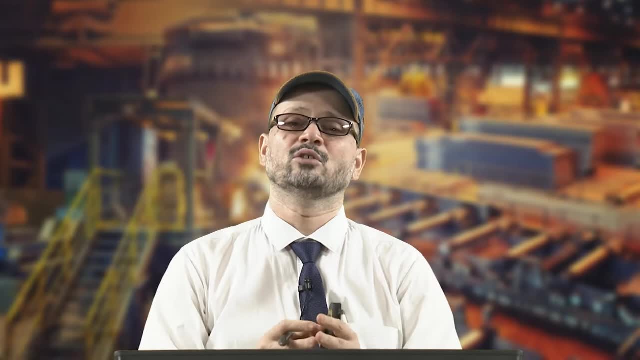 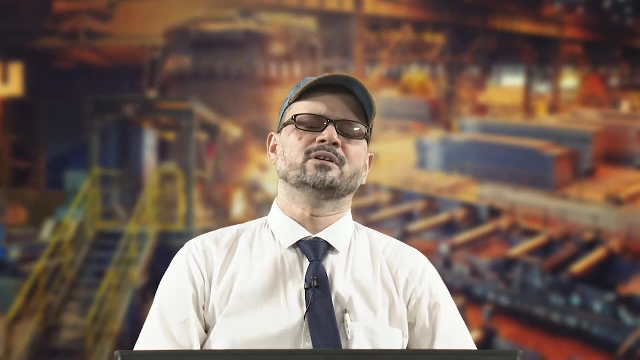 So you may go for two grids. So you may go for two grids, So you may go for a 2D structure or you may go for 3D structure. So, based on that, you know if you have the 2D type of grid. 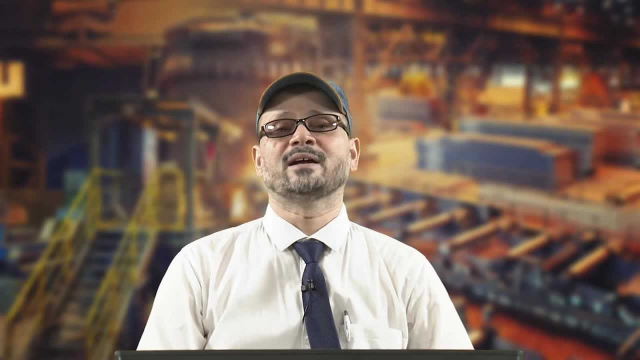 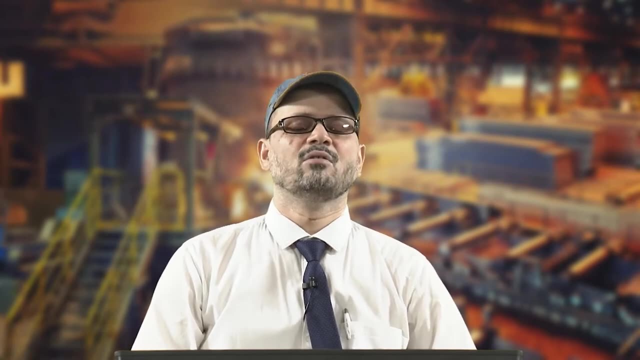 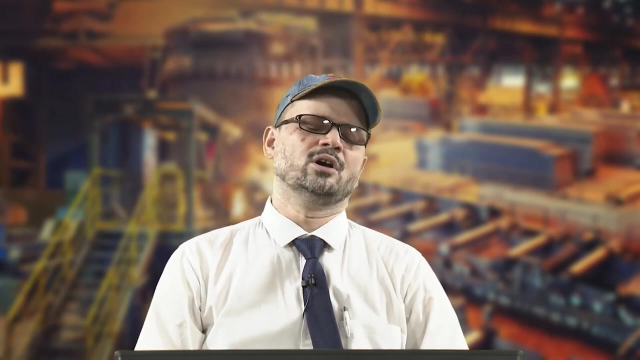 So you have, you may have the element type, maybe, like you have triangular, or you may have the quadrilateral type of element, whereas if you go for the three dimensional ribostructures you have different kind of- you know grid topology, So that may vary from the Name. 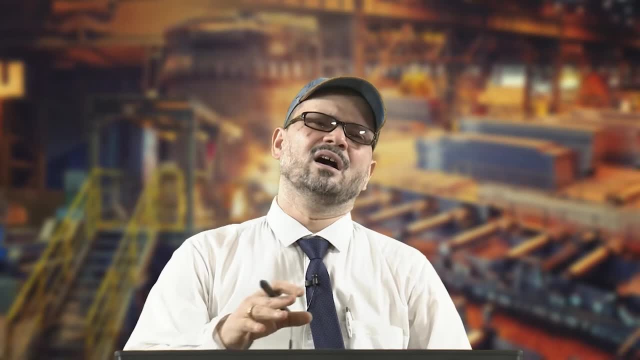 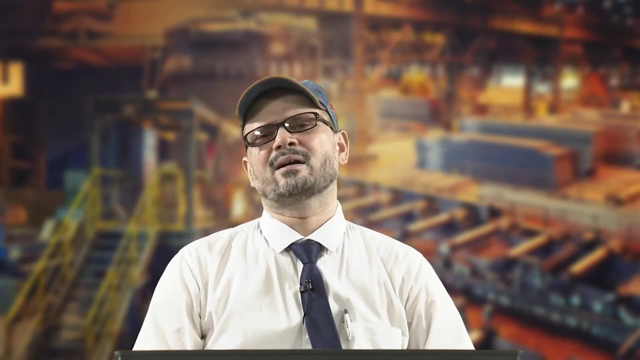 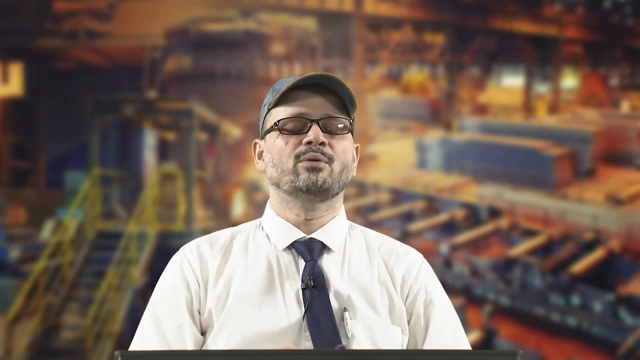 from the tetrahedron to hexahedron to, you know maybe, prismatic type, So you have different kind of, or always shaped, So do we have. may have different types of elements which you may choose when you are making the grids, Then you know approach of making the geometry. 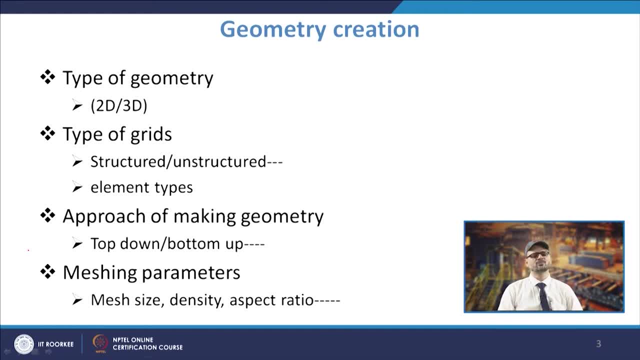 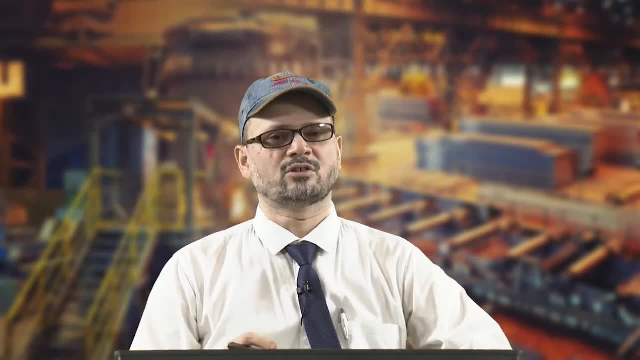 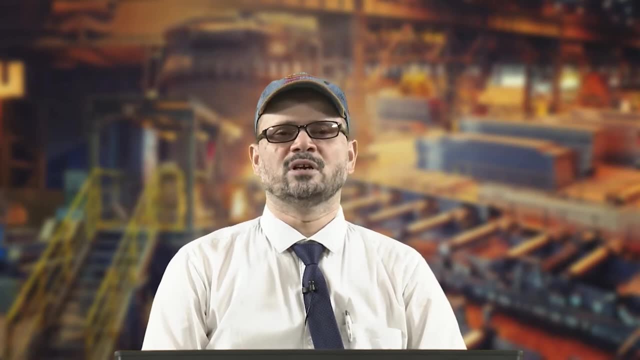 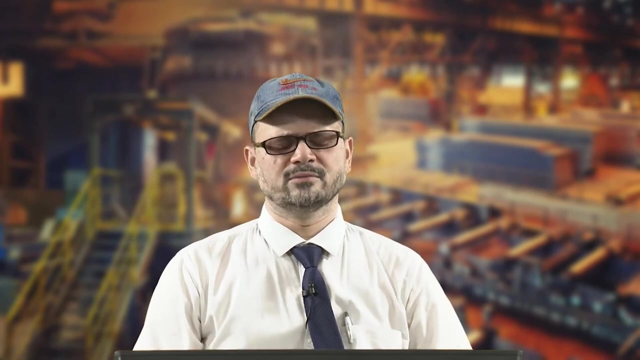 Now here you must know that you can make the geometry in a top down or bottom of approach. So this is normally available with the commercial solvers. So you have many kind of commercial. you know CFD tools like phonics: fluent is there, star cd is there or there are many. 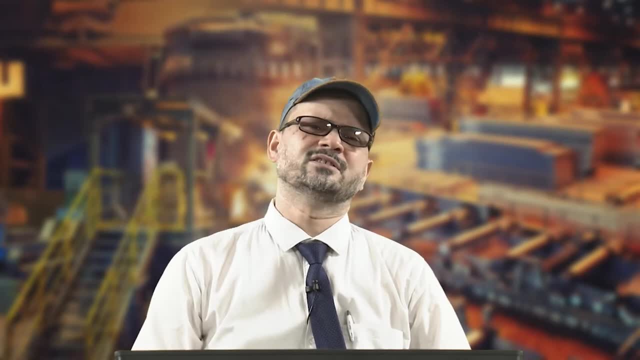 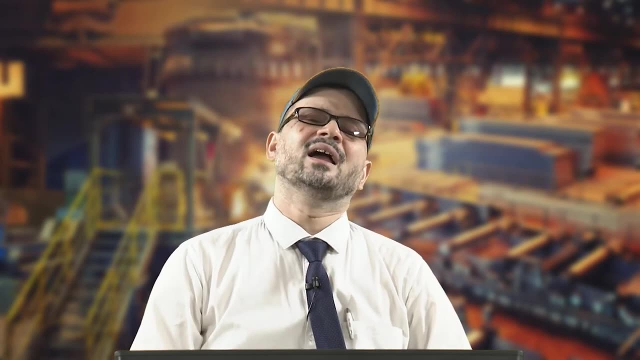 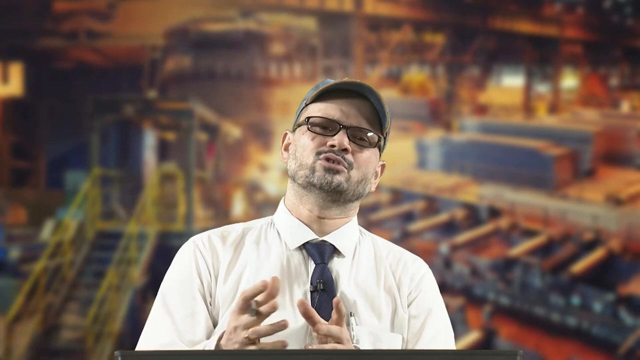 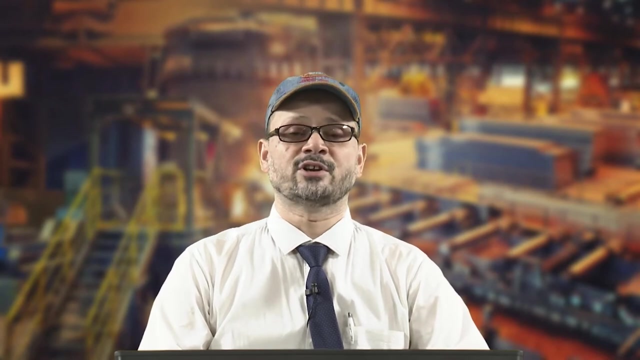 you know CFX and you know all these, So these are So using their in their own way. they are making the geometries and you know you have solid modeling tools also, like you can use the solid modeling tools, solid works and all that, So you can use the, these tools to make the geometry. Now, making the geometry is using. 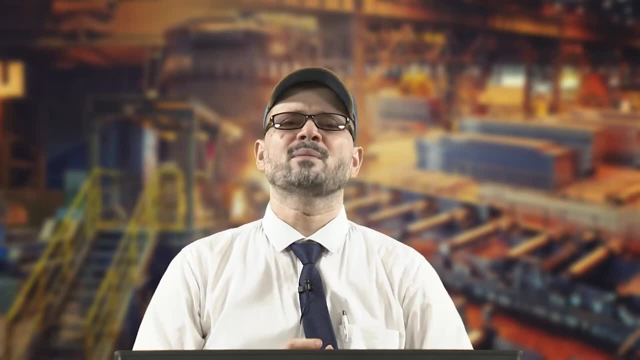 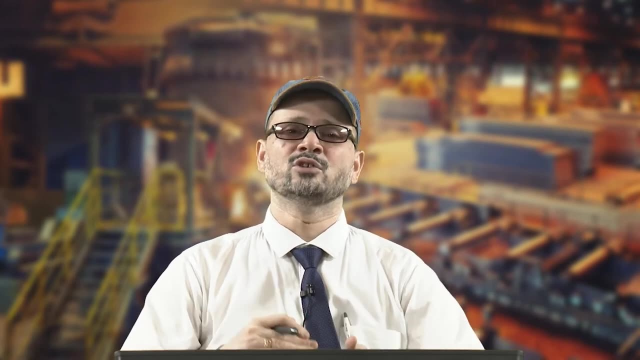 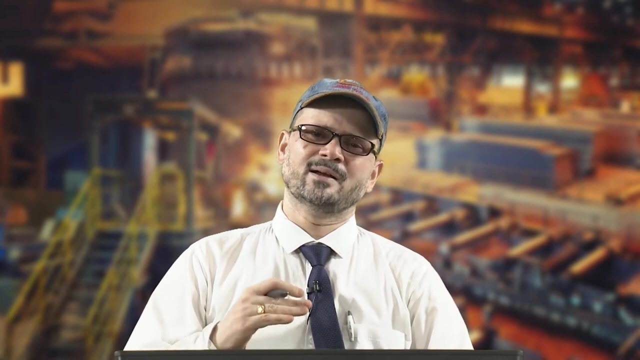 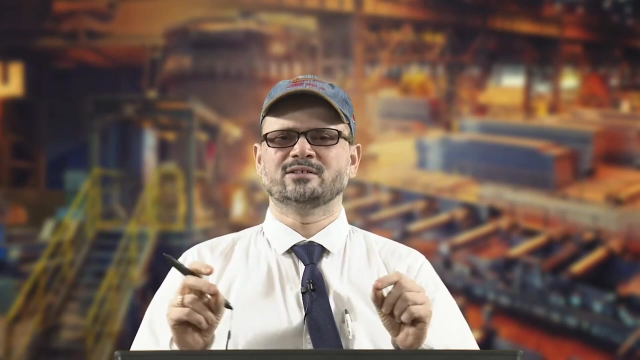 the top down or the bottom up approach. So bottom up approach means you are starting from the initial and then making The things and moving towards the final result by adding by in, the adding stepwise, addition of stepwise. Like you are first of all making the points, then you are make joining the points. 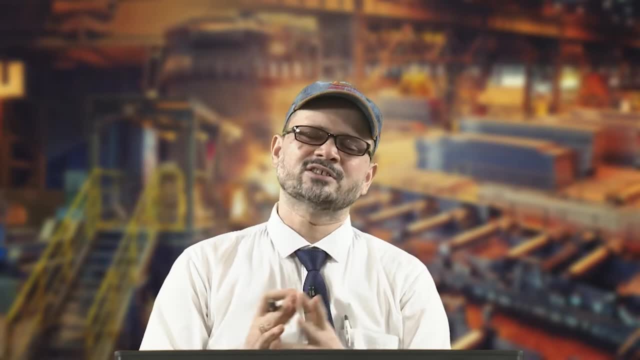 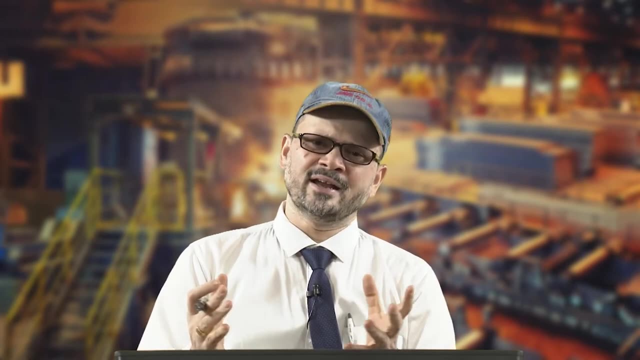 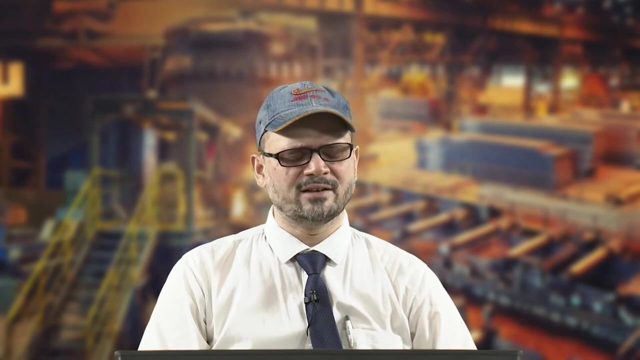 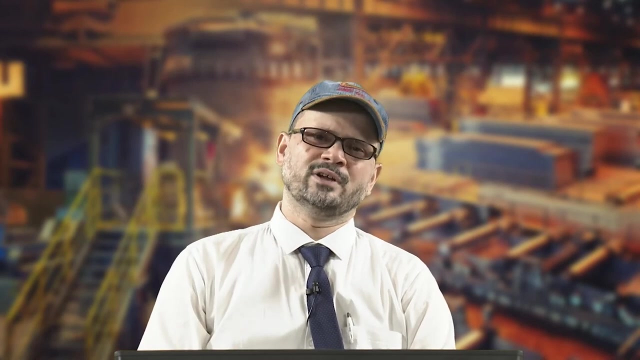 that is, by lines, then you are making the faces, Then you are making, using the faces, you make the volumes And then you integrate them and then, in that you may specify a certain kind of- you know- zones, like you may have the blocked zone, where you want that it should be blocked or so, or 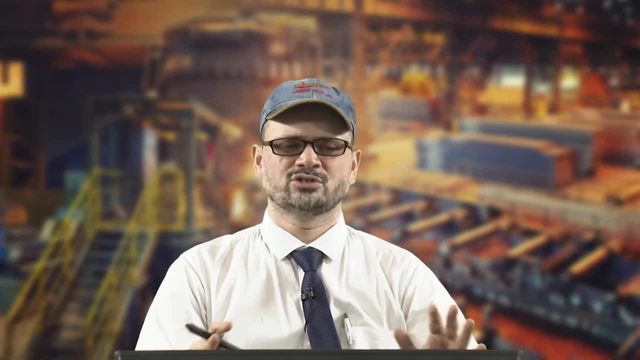 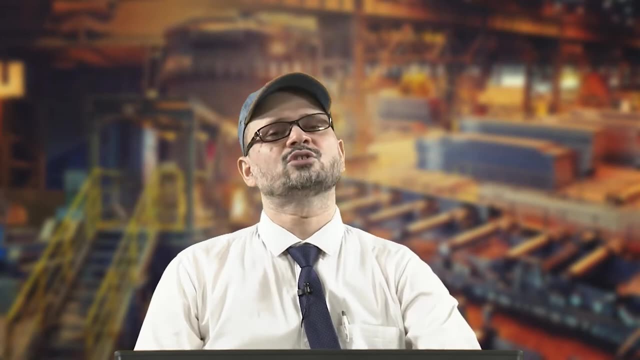 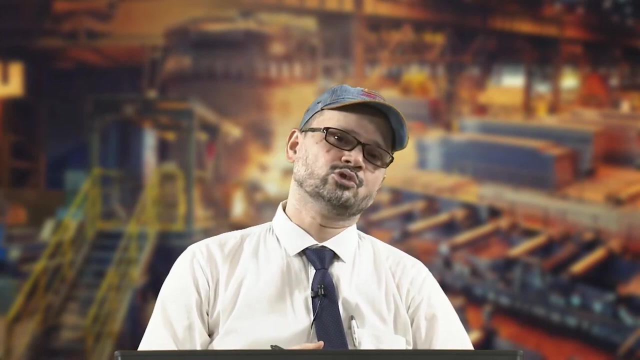 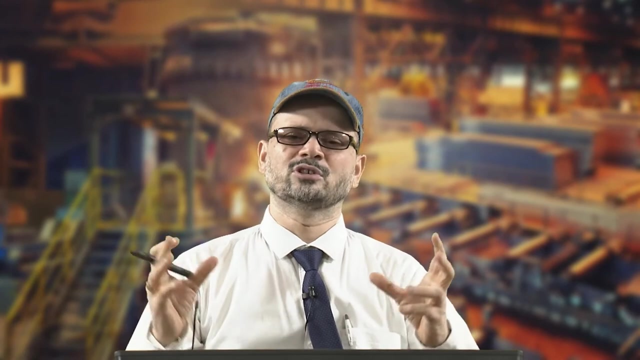 you can specify there itself other zones So that we will see like different zones, like wall inlet or so. So that is top bottom up approach. In many cases we go for the top down approach also, like you know, many a times it becomes helpful if you have to make, suppose, one geometry, suppose 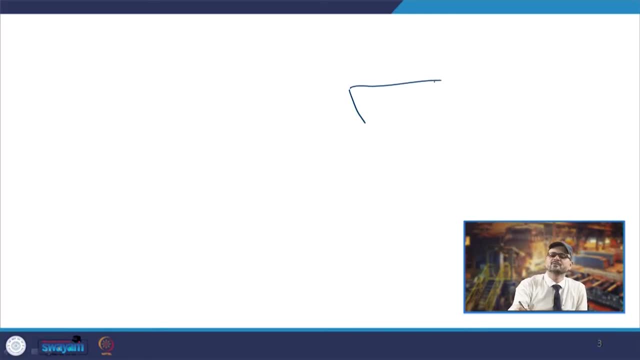 you have to make a geometry where the things are suppose this way, that is, you know, tapered, So in that case you can make one geometry of this type and then maybe that you can take this part being off, So that is, removing this part, taking away, So that will lead. 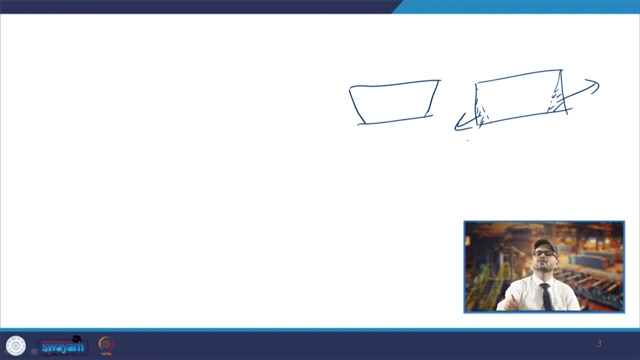 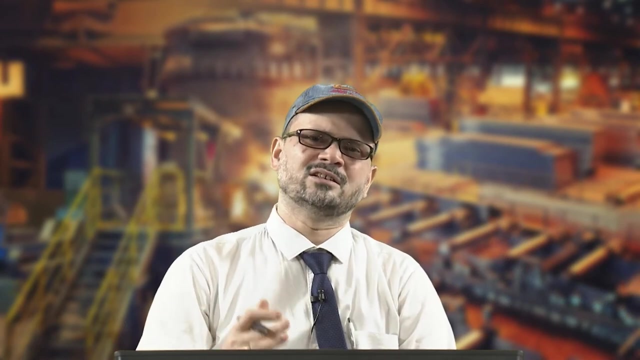 to this result. So you can start with a rectangular type of or a you know, three dimensional structure and then cut a certain portion and make the required geometry. So that is bottom up- I mean top down- approach. So you make the larger, you know geometry, and then you are, you know, reducing that and 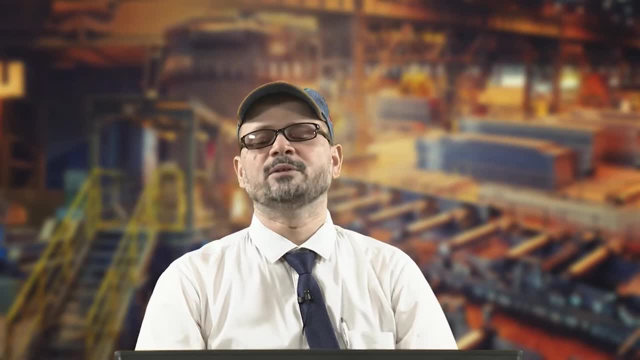 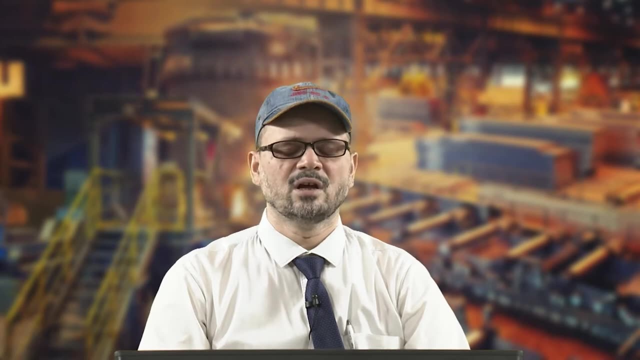 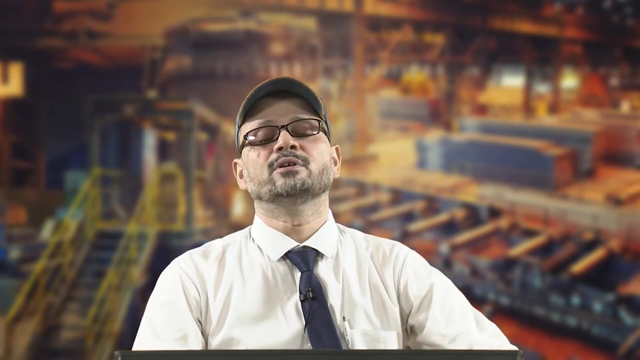 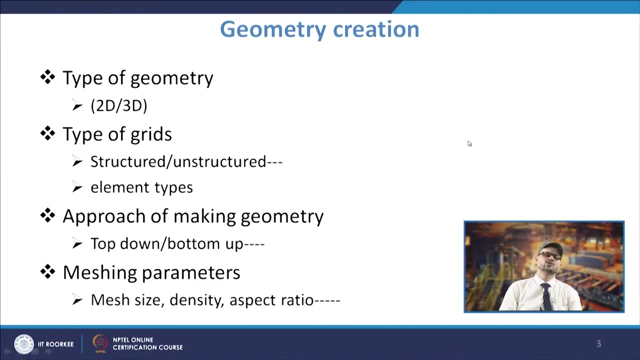 getting the required geometry. So that is using the top down approach. So both the approaches basically are you know in practice and used by the modeling tools to make a proper geometry. Then comes the meshing parameters. So once you make the geometry you will be making the 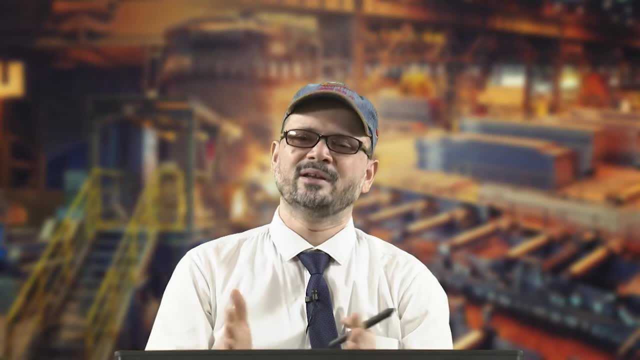 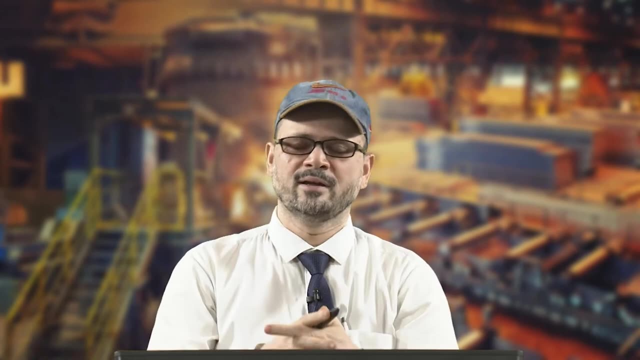 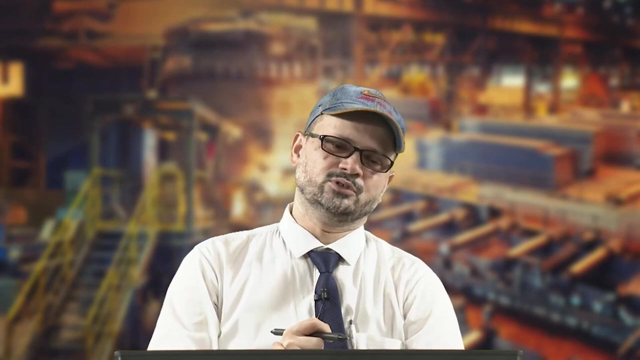 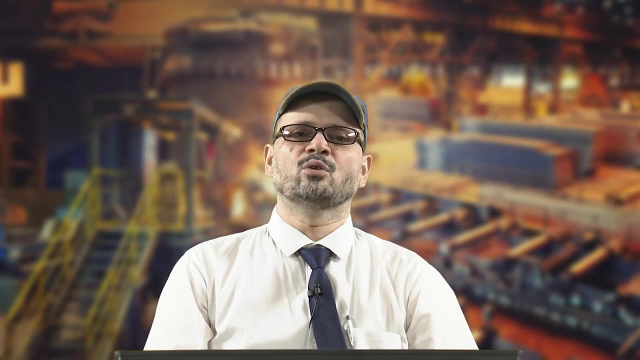 geometry. you will be integrating them. you will be making a complete, you know geometry of which will be physically representing the domain. Then you have to go for the meshing of these you know geometry. Now why meshing is important, that we know that by meshing we are going to have the formation of the small control. 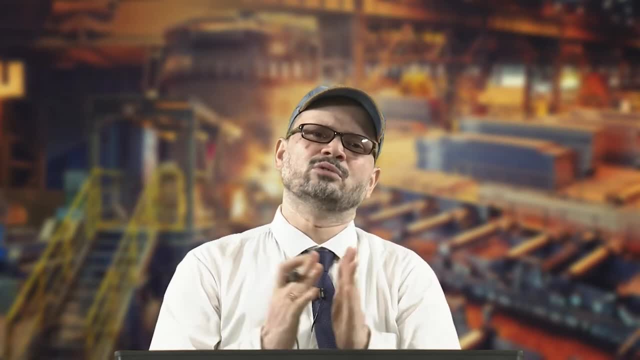 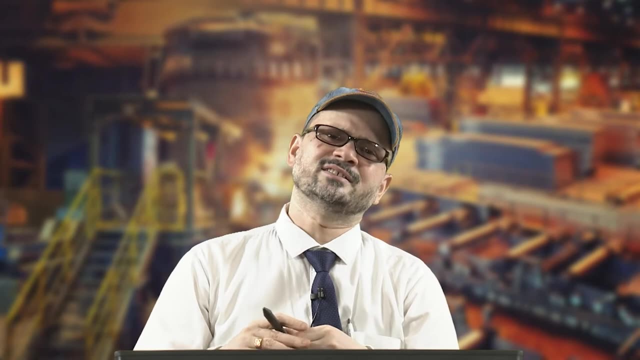 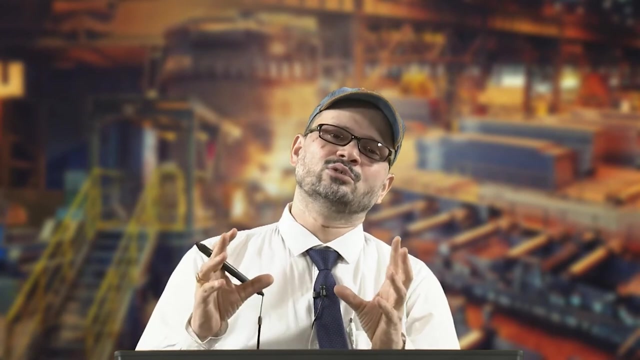 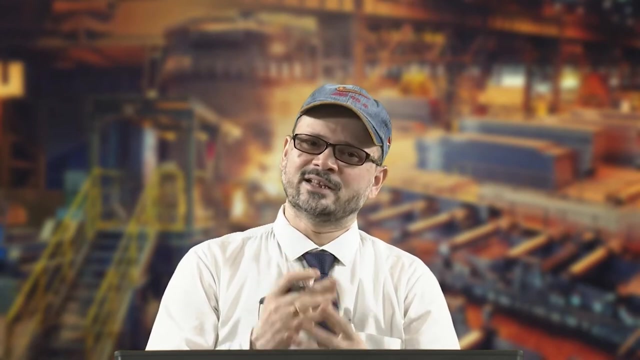 volumes or elements which will be linked to each other, So that when we apply these conservation equations and solved, you know when the equations are solved simultaneously. in that case you are going to have the values of the you know parameters or variables. So these are the values in the respective cells or at the respective nodes. 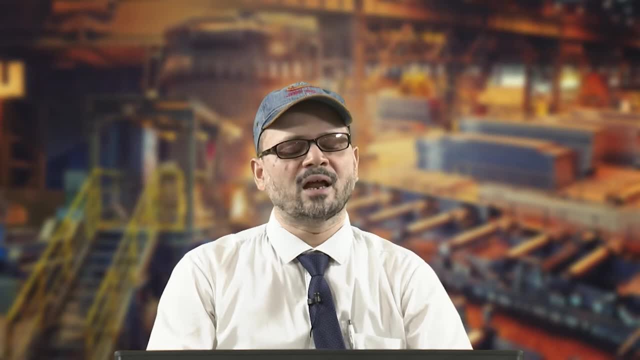 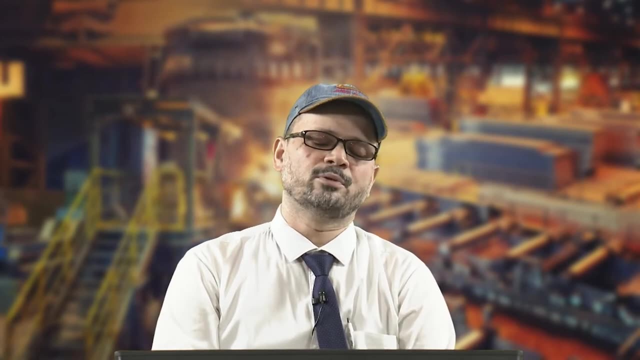 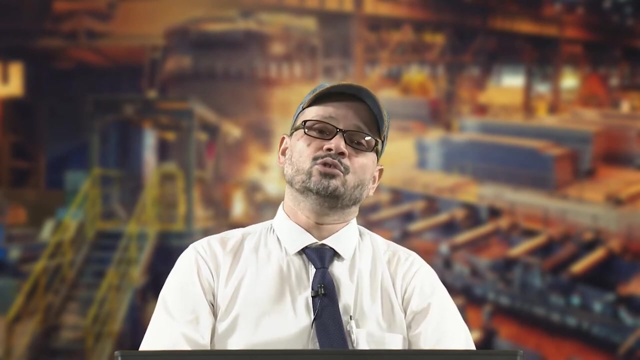 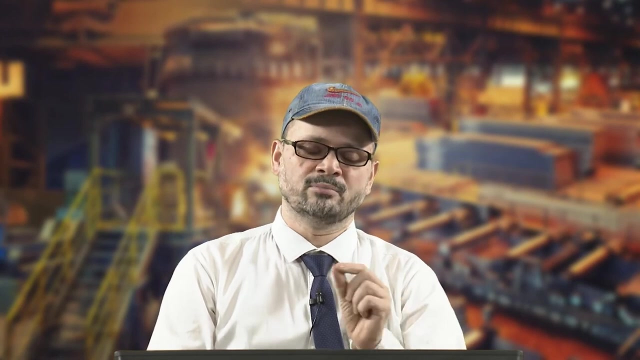 So the meshing needs to be done properly Now, while meshing you need to have the you know proper, you know care for the mesh size So you can have the large you know number of meshes. So if the mesh size will be small, you can have a small number of mesh. So mesh size 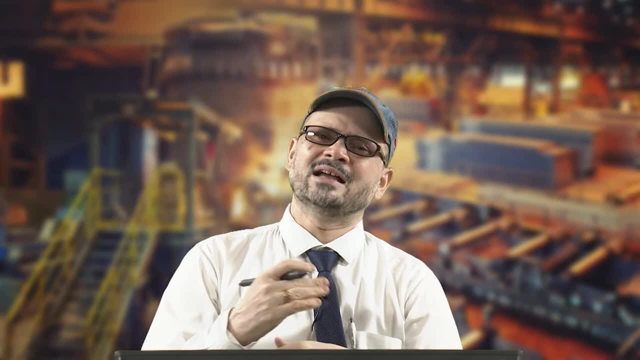 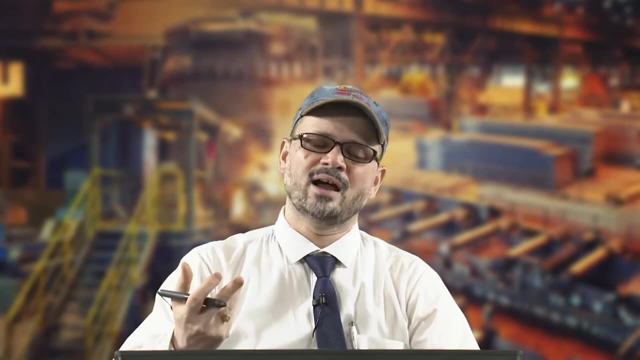 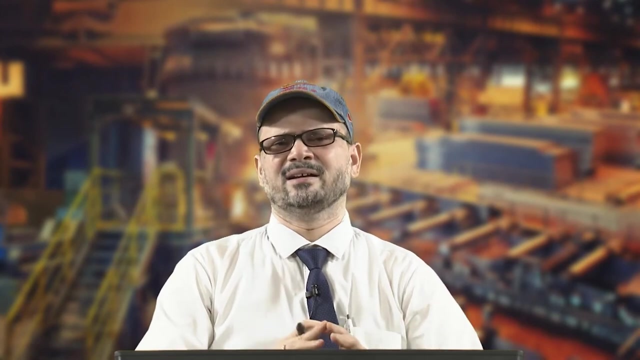 will be larger. Now, every you know, as it is quite evident, that when you take large number of mesh, in that case the computational time will be higher, and when you take less number of mesh, the computational time will be lower, but then certainly the accuracy. 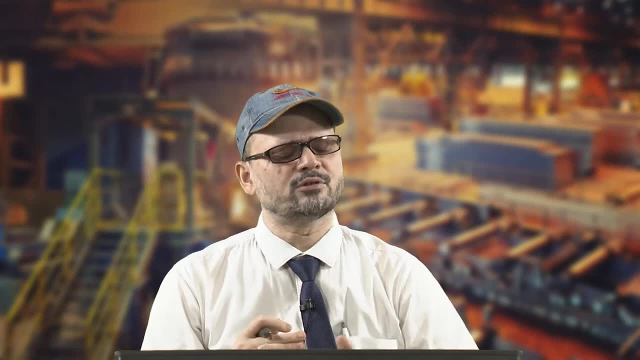 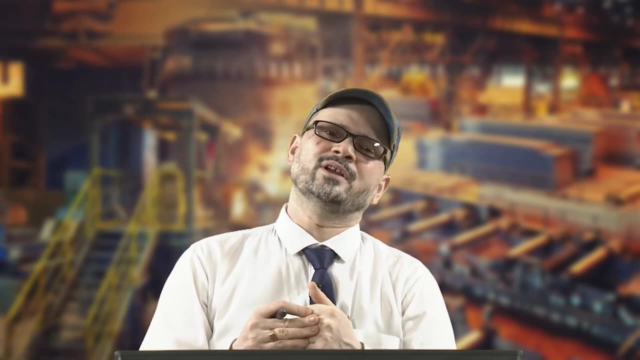 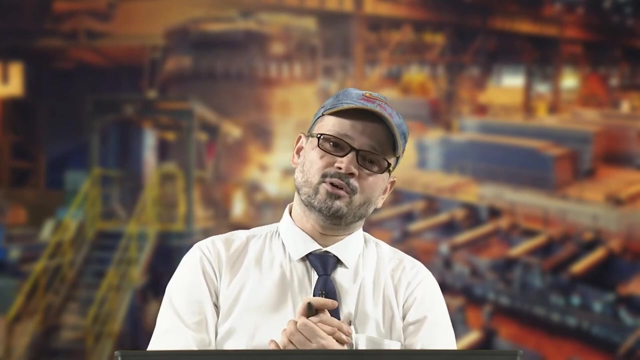 will be affected. So, accordingly, you have to take the mesh size. You have also to be careful while taking the mesh size. what should we? what? by what way? the, even the mesh size, should vary. So in case of the boundary layer regions, you 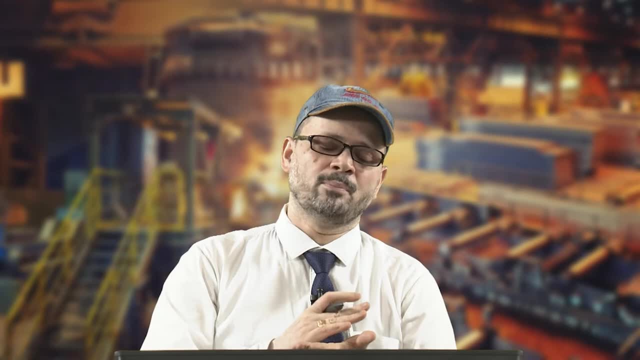 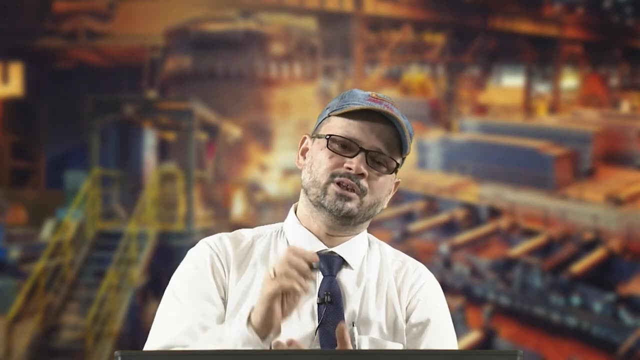 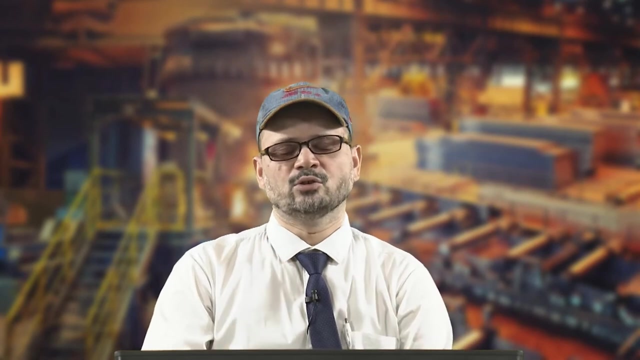 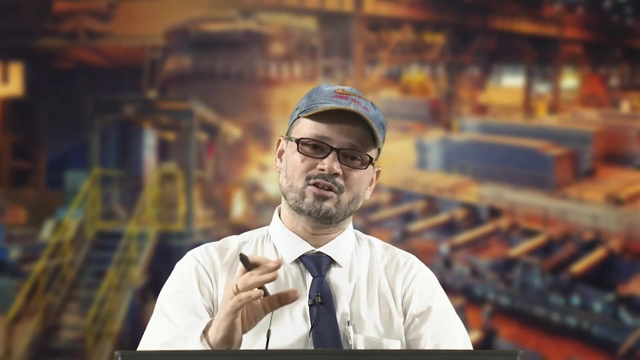 may have to have the- you know- proper variation in the size of the meshes from the walls to the point in the active domain, So that to basically properly- you know- predict the output parameters. you need to have a an understanding of that also, that how you have to maintain. 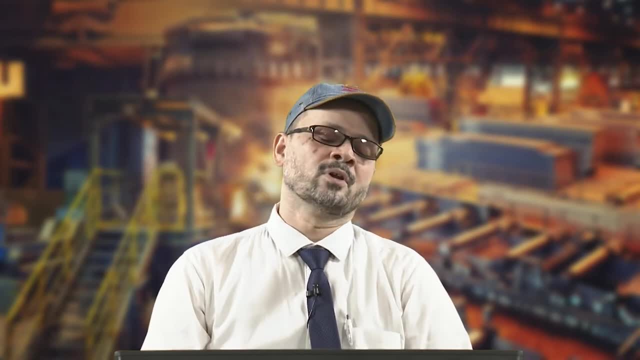 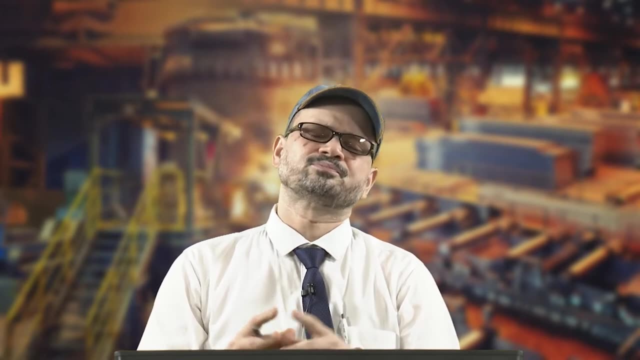 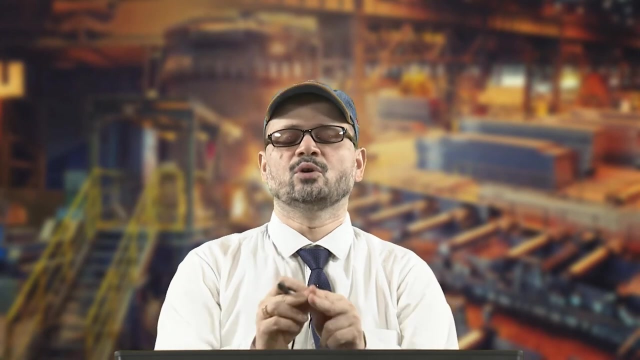 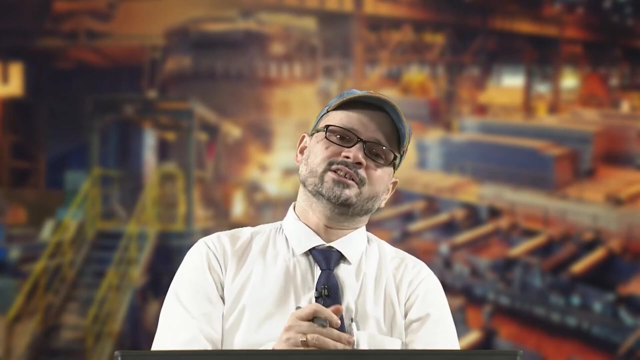 those you know mesh size, Then the density- that is what it talks about- and also the aspect ratio. So typically you know aspect ratio will talk about the you know ratio of the dimension of the you know mesh in the particular directions. So basically, 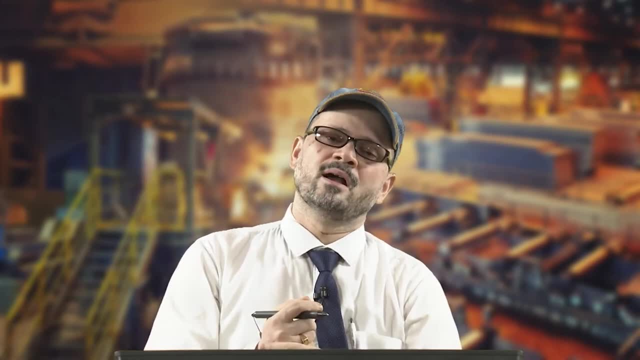 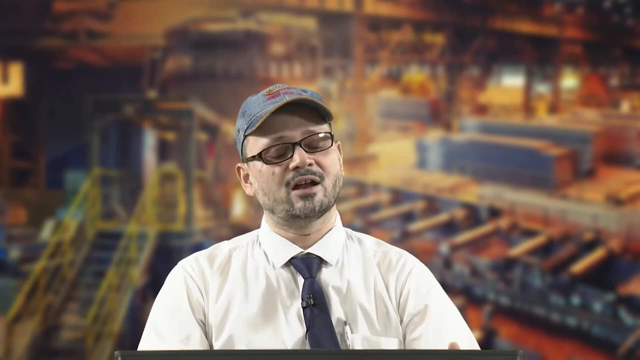 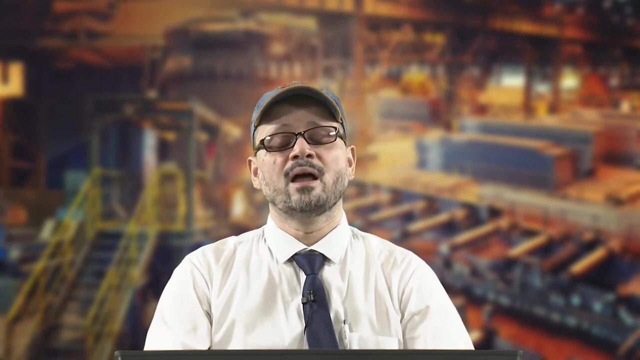 we try to have aspect ratio of 1 normally, which is more ideal, but it is not always possible, So we try not to To have a very large value of aspect ratio in most of the cases. So these are the you know points which needs to be looked into while going for the meshing. So once you 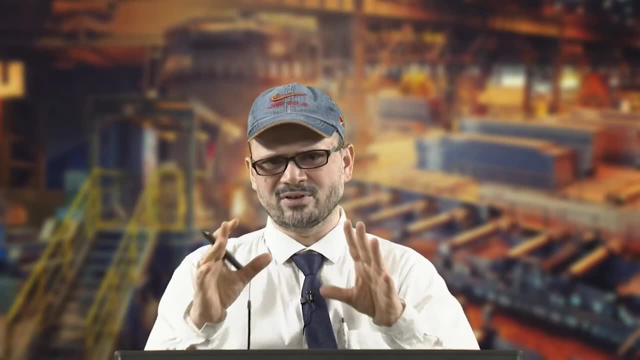 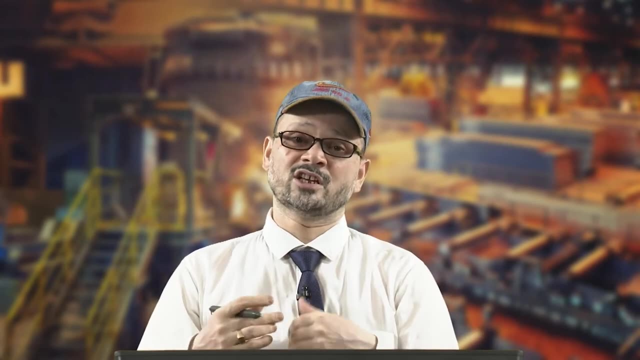 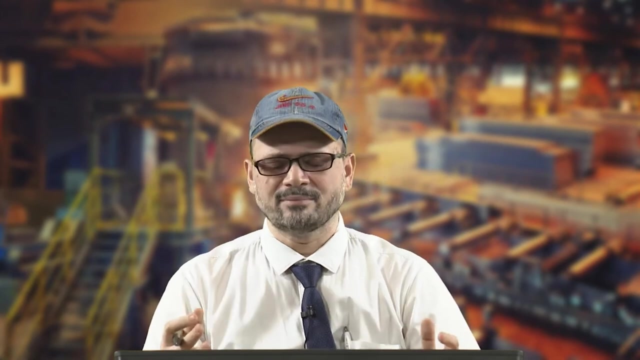 do the meshing, then it will show and you can have a look of the mesh- that how the meshing has been done. So you have to go for the checking of also the meshes and you can. Then the softwares have the capability to ensure that there is proper mesh. Otherwise, 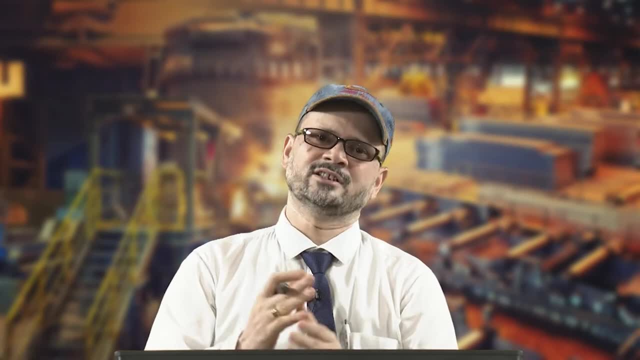 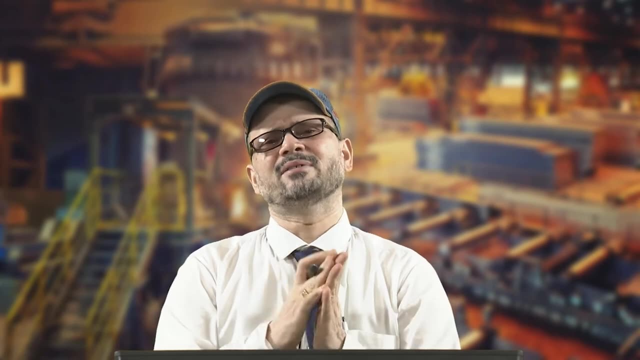 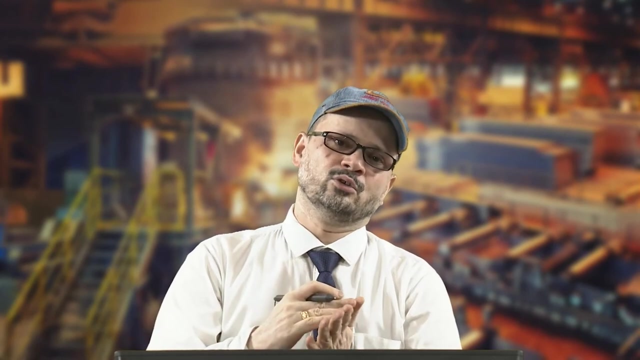 they may so tell that there is no proper meshing, there is no proper integration. Maybe once we the situation may be such that you have done the meshing, but there the portions are not integrated, So there will be two different zones and there may not be, you know, transfer. 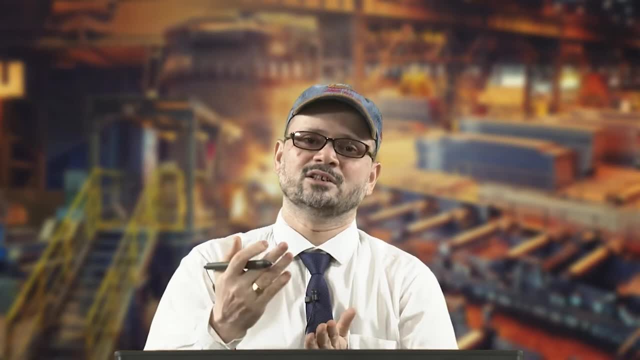 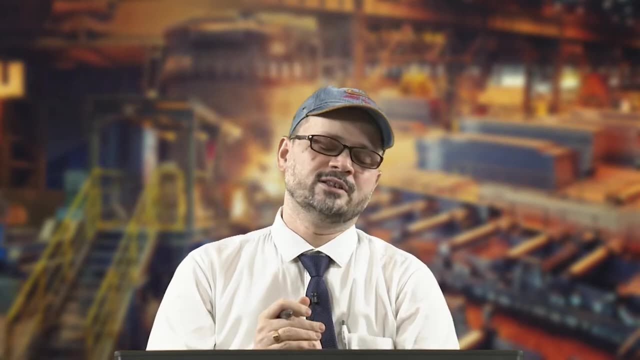 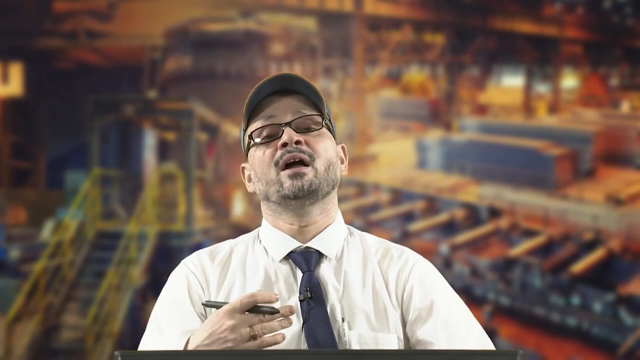 of information from one region to other. So all these things need to be checked. So you need to be checked into while when we do the final meshing, at that time you need to check all these things So that you can go further. and when you go for specifying the other parameters in the 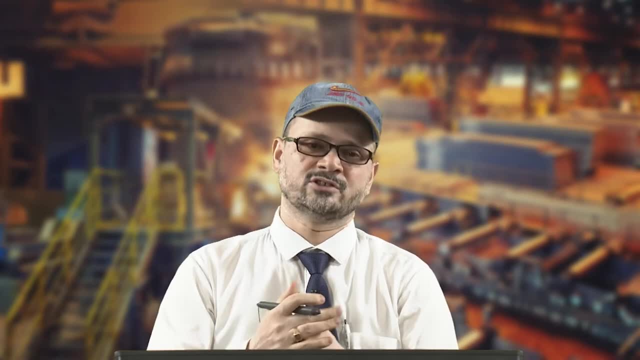 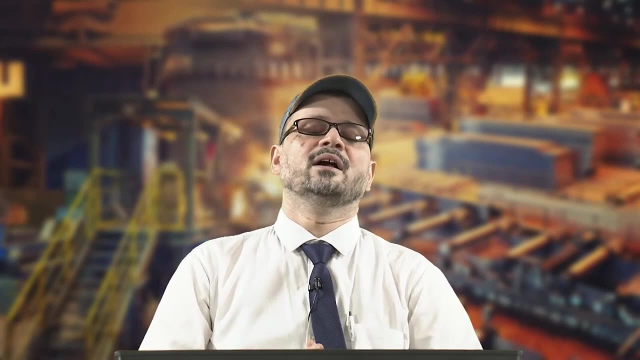 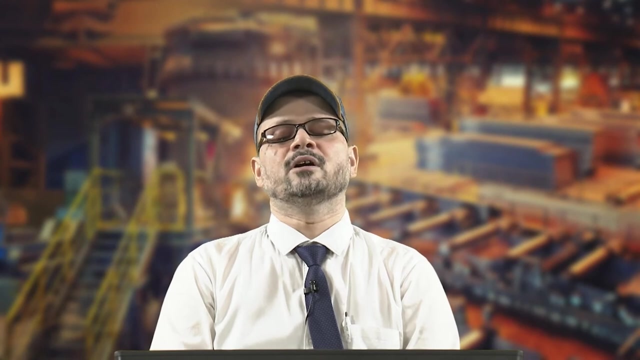 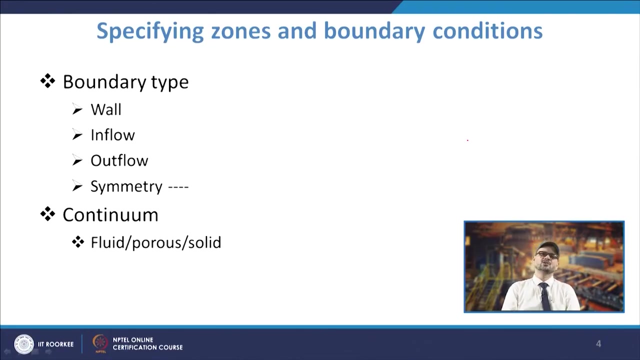 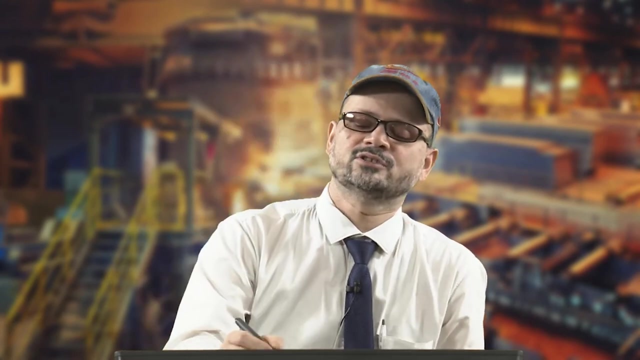 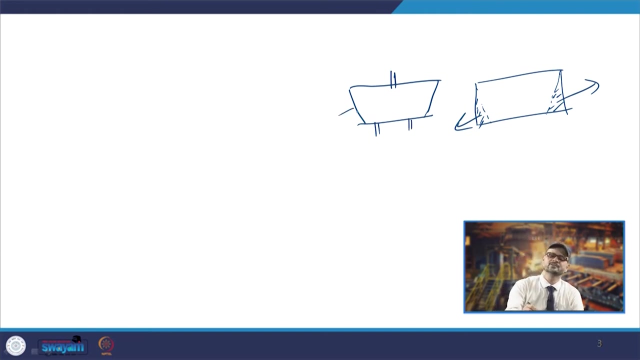 domain, so that time you have not to face much of the problem. So, after the meshing, or and after the some of the tools you know, while making geometry itself, you can show them as you, you, you show them as the walls or the blockages, And some of them, while providing the solution. 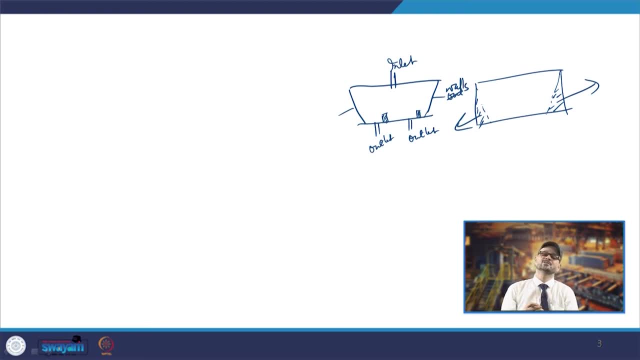 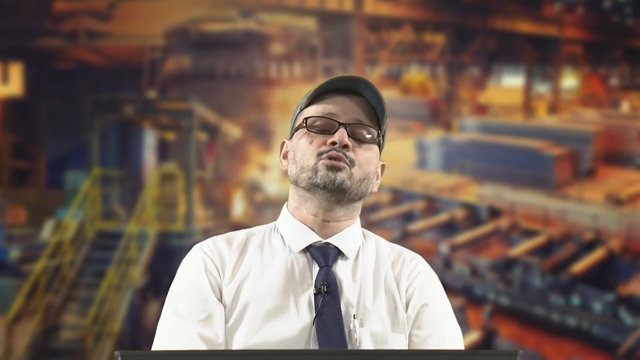 control parameters or while giving the boundary conditions. there you have those, you know, options where to define that this is wall or so, And then, accordingly, you have to provide the proper boundary conditions. So, if you look at the this, So what you have to do is, first of all, you have to define the zone where you 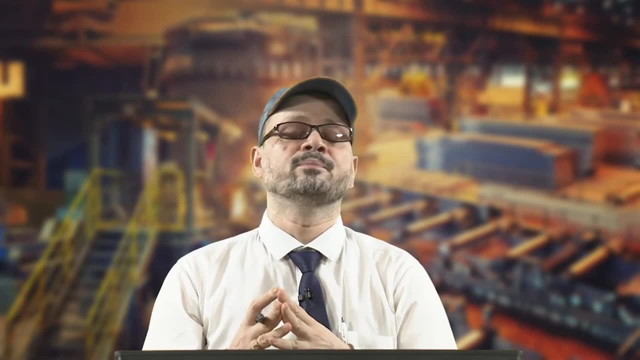 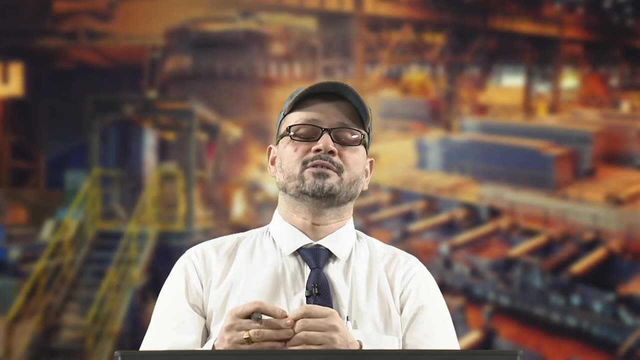 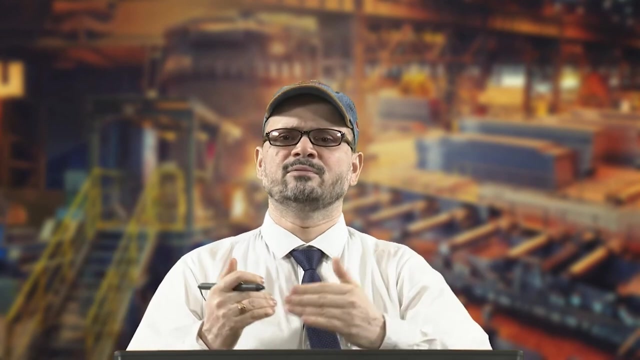 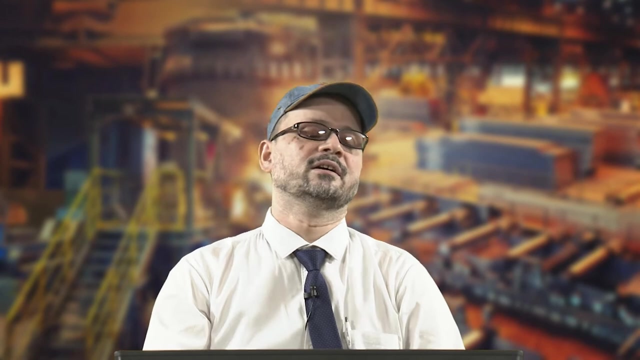 define the boundary type and you also define the continuum that is. So in boundary type, normally you have the, the boundaries you know, specified in terms of walls, because external boundary is normally the wall. So you will have to define those surfaces as the wall. Similarly, you will have the conditions like the inflow, So you 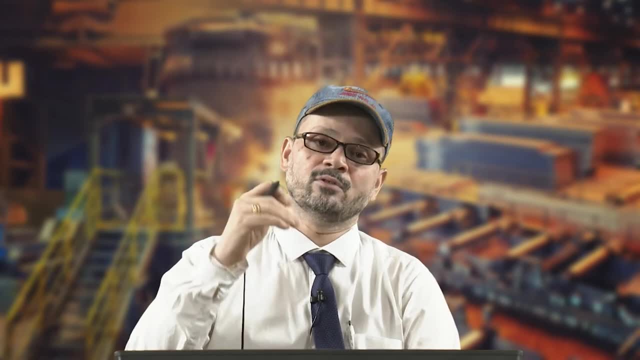 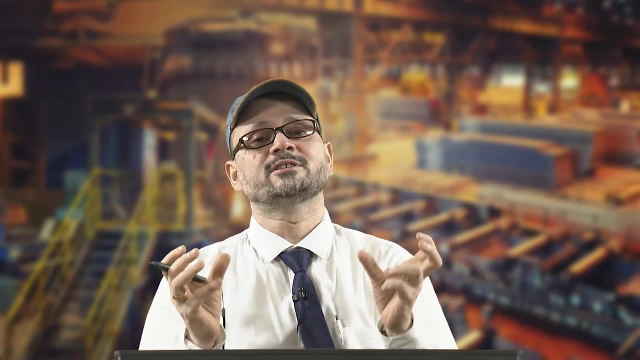 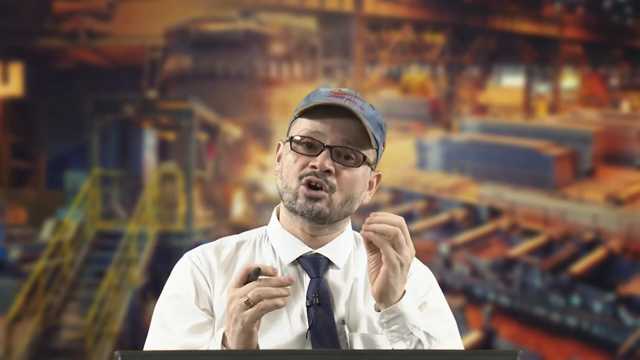 will have inlet, So that will be the inflow boundary condition will be there. then you have outflow boundary condition, that will be outlet. So basically, while making geometry also you can specify those zones as As the walls or the inlet, or inflow, or outflow, flow or symmetry, So it will go there and 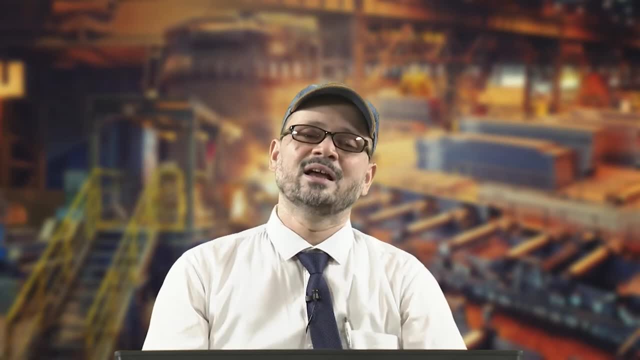 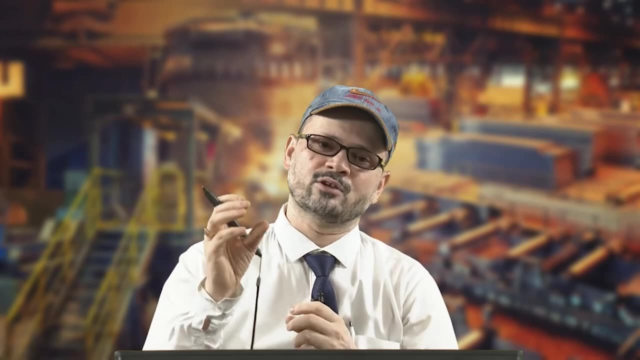 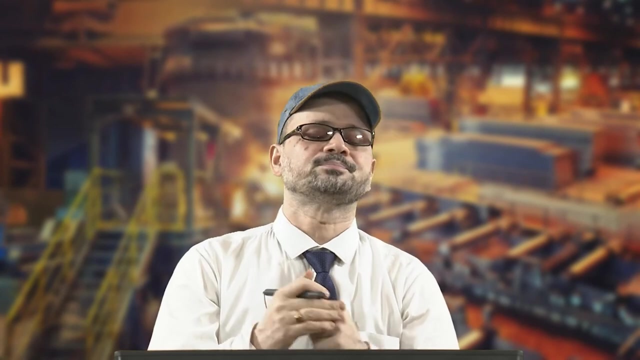 while you are giving the proper boundary conditions. at that time you can have the selection from the you know drop menu that if you take wall whatever you have specified as walls, they will come and, properly selecting them, you can have the proper values fixed to them. 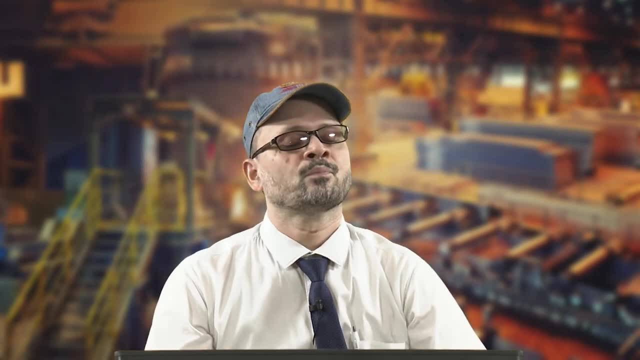 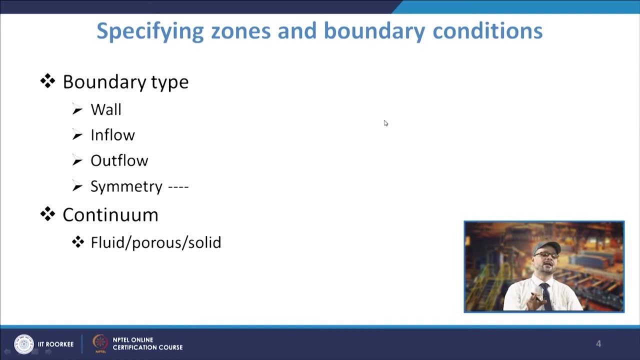 So you know, this way, you provide these, you know, you specify these zones as the boundary types and then you are going for the continuum or the you know. So in continuum, you know means that you are going to define the domain wherever you have the fluid. So you will say: 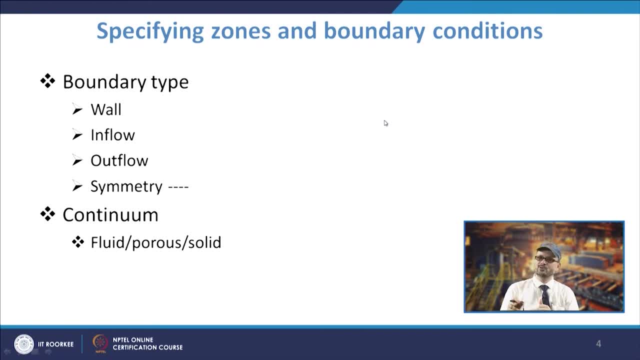 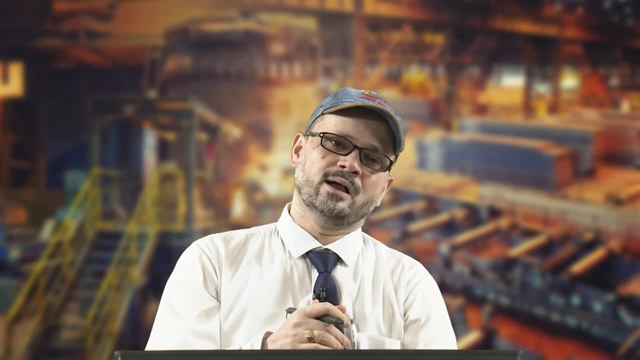 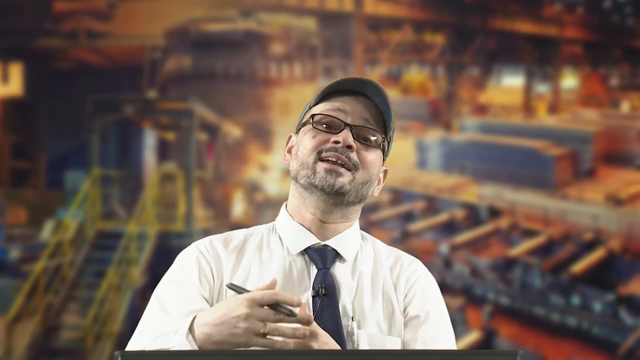 it is occupy, going to be occupied by the fluid. Similarly, wherever you have the existence of porous materials- in case of porous, you know flow, So you have to define that. this region needs to be specified as the porous material and, similarly, if there are blocks. 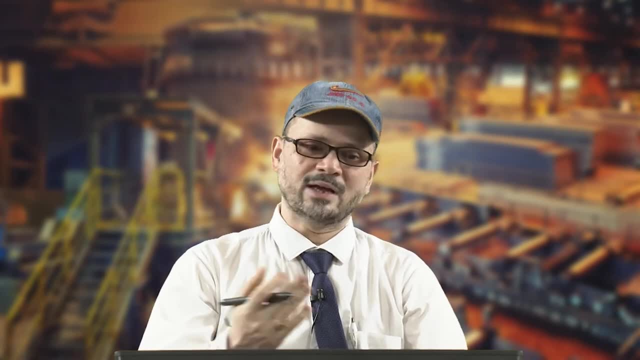 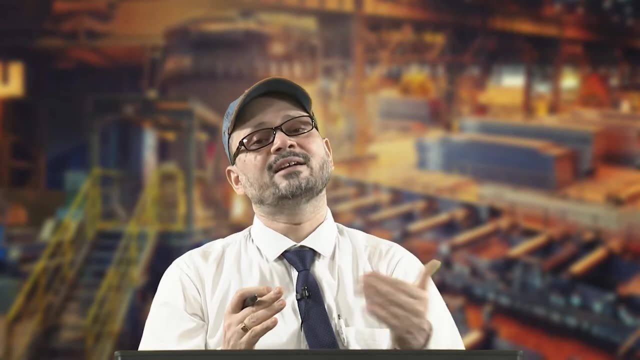 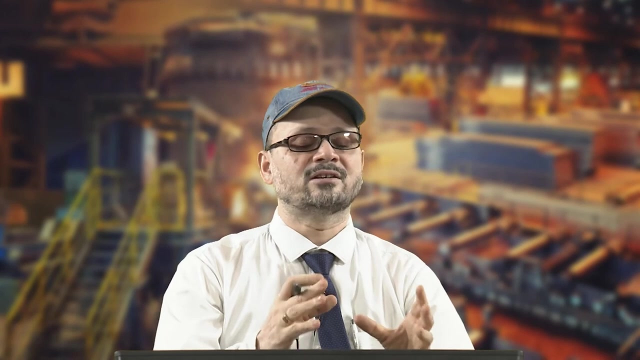 or solid portions, So you need to define them. So, as I told that you can define these things, either while making geometries, or you can and there itself, or while you are specifying the boundary conditions. you can do that job, you know, while going for the specifying the. 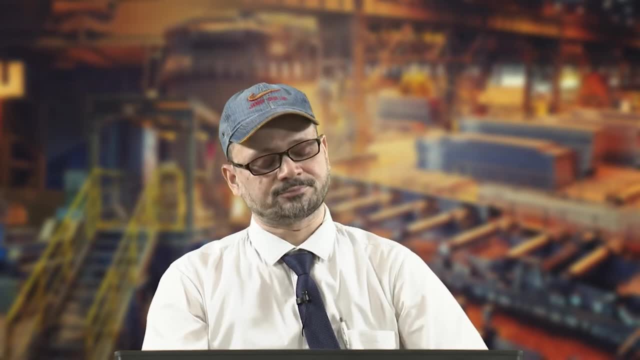 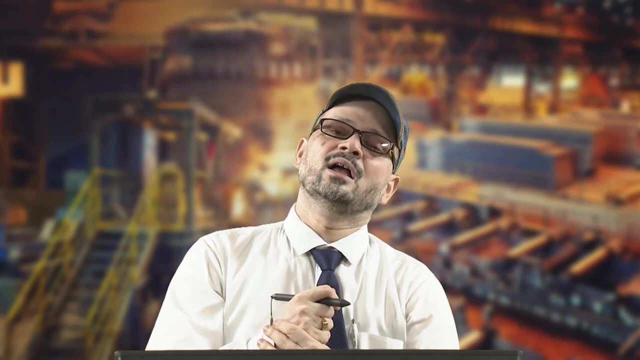 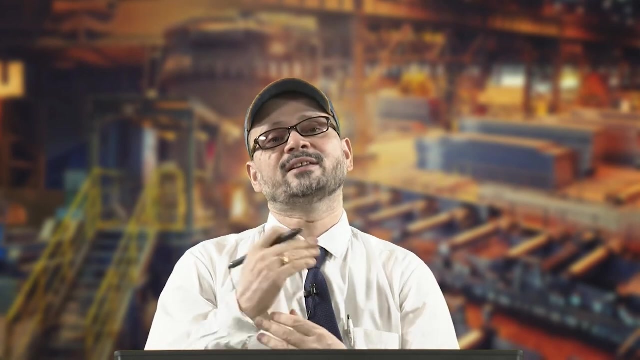 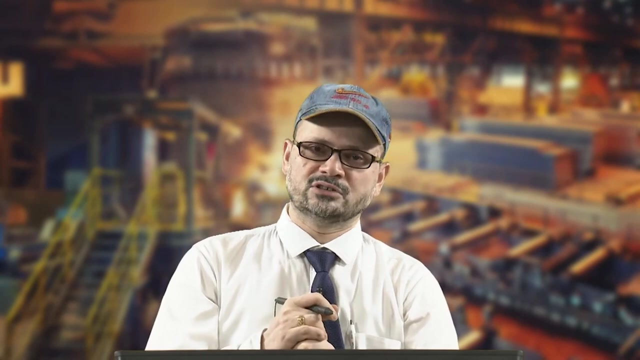 zones and the boundary conditions. So once you have given So those specified these zones as boundary types, and also the continuum, that is, where there is fluid, where there is solid or so porous media, then you have to provide the solution control parameters. Now, solution control parameters means now, after that you 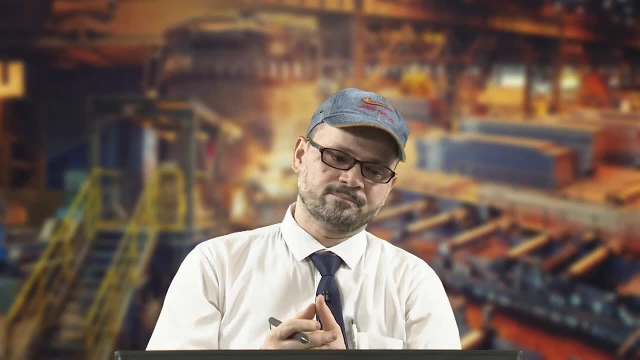 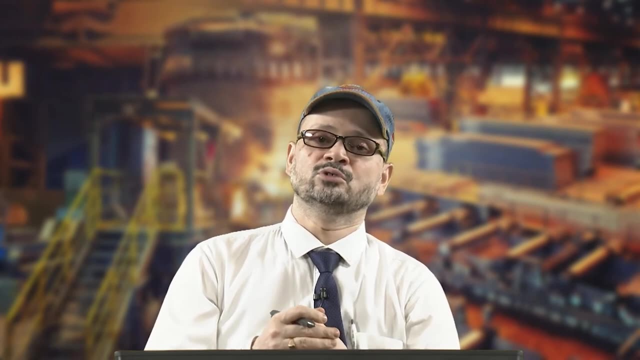 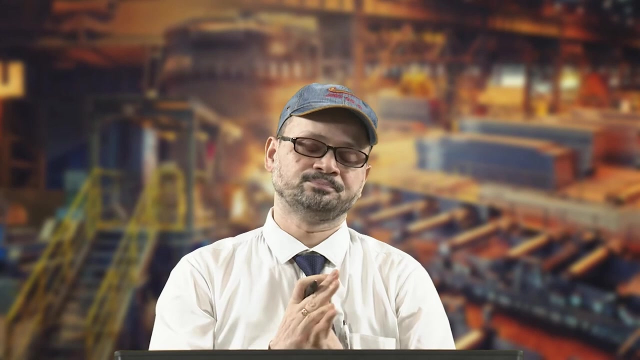 are going to have the solution started. Now, what you need for need to specify when you have to. you want to talk about the solution to be started. So basically, you have to tell that whether your solution is steady or transient. So if it is steady, it is fine, you have to. 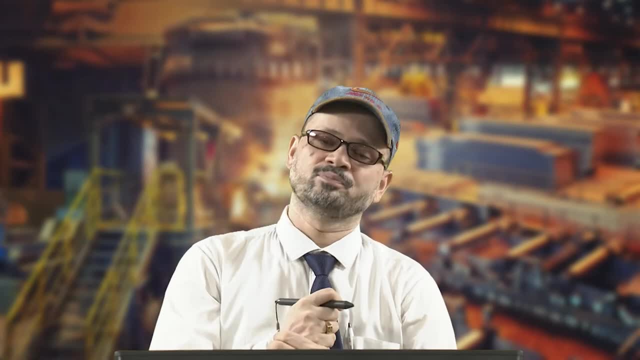 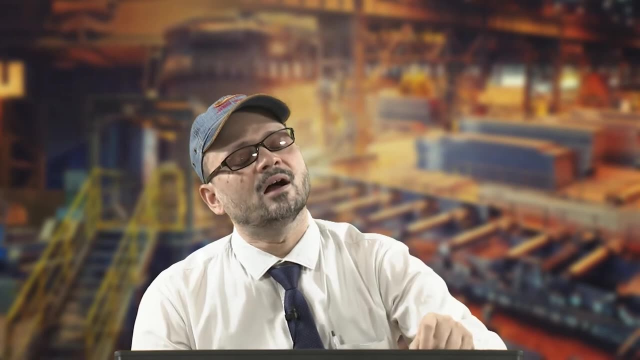 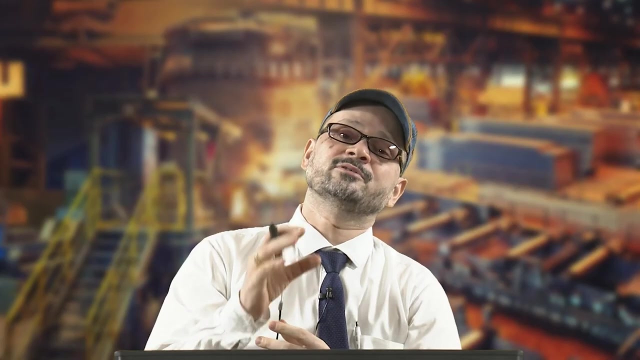 tell that for how many iterations you are going to stop. after how many iterations you are going to stop and see the result, Whereas in the case of transient analysis you will have the specification of the time step sizes. So for in a particular time, depending. 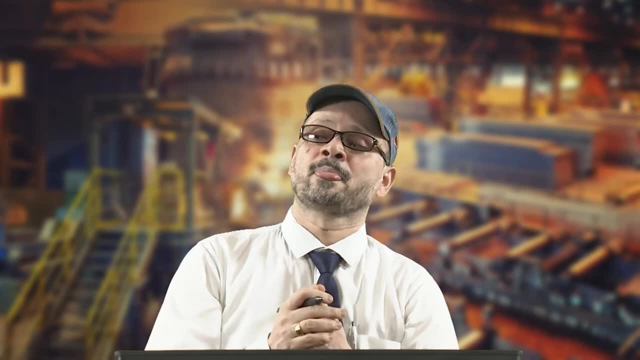 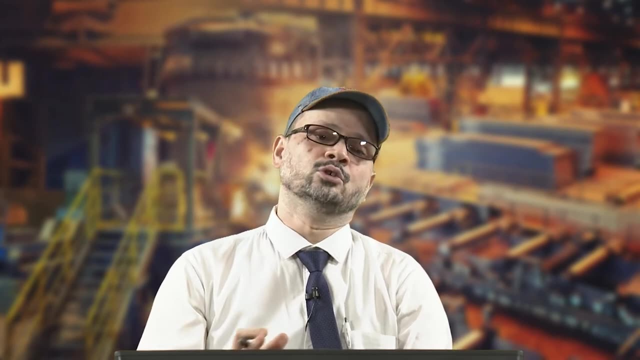 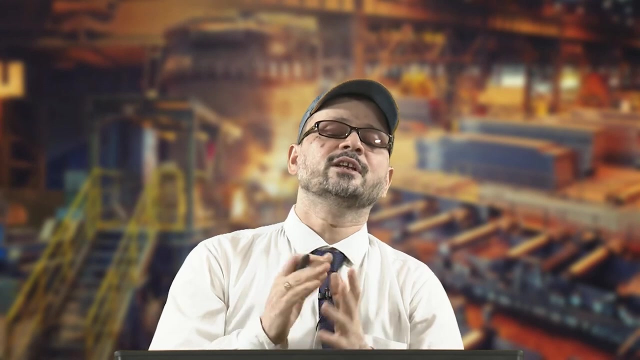 upon the step size you will go. it will go for that many, you know number of iterations and you are going also to provide certain relaxation parameters, So that parameters need to be specified, you know, towards getting a converged solution. So these, you know, relaxation- 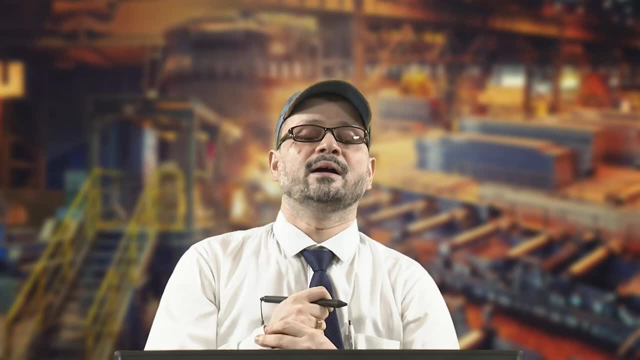 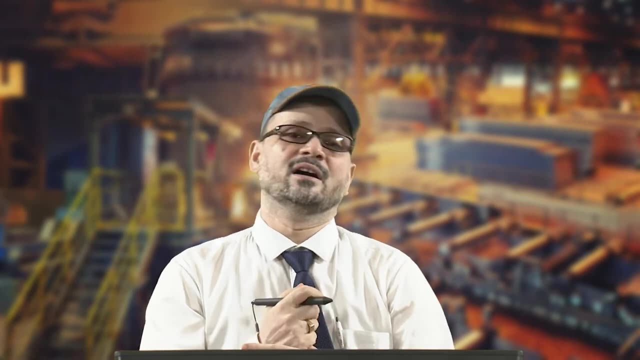 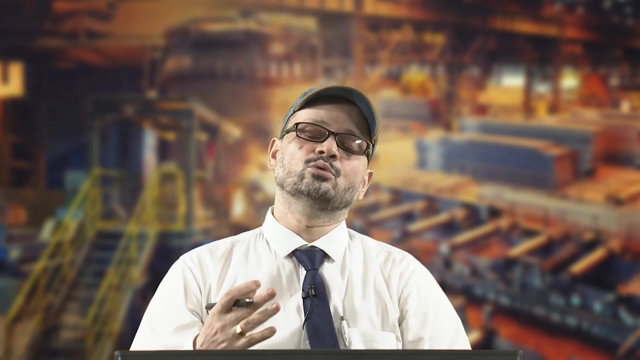 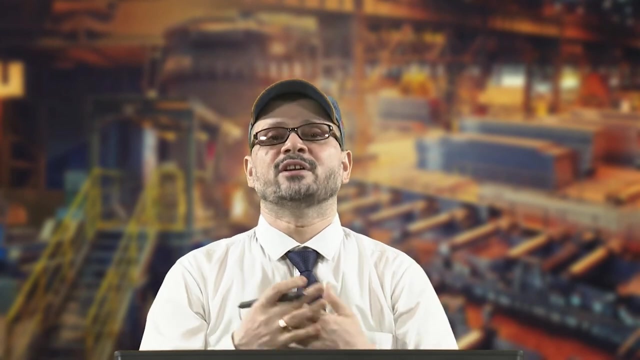 parameters will be provided And then the solution will start and it will reach till the till you get the results. So once the solution is over, in that case, after that you go and do the you know post processing of results. you interpret the results in your own way.